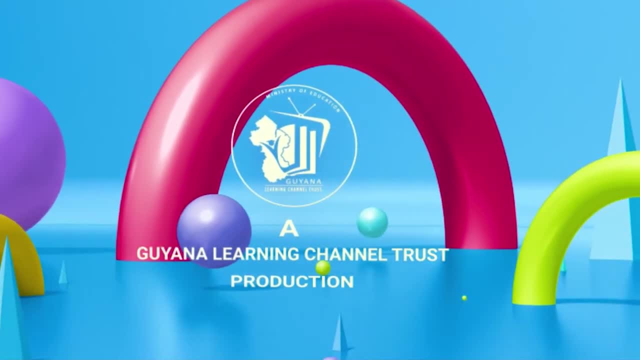 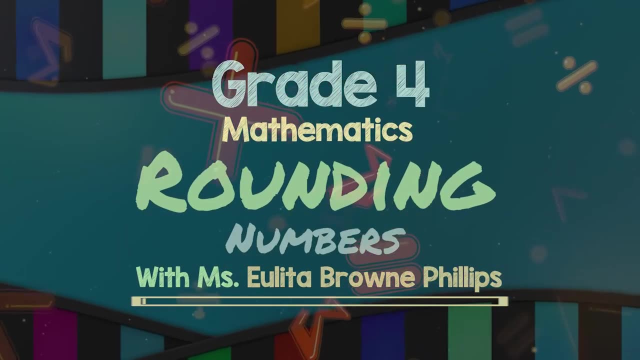 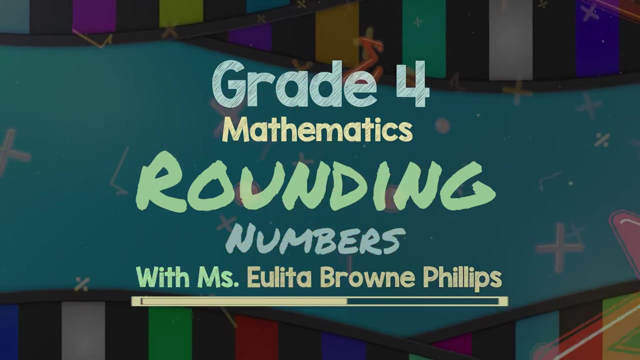 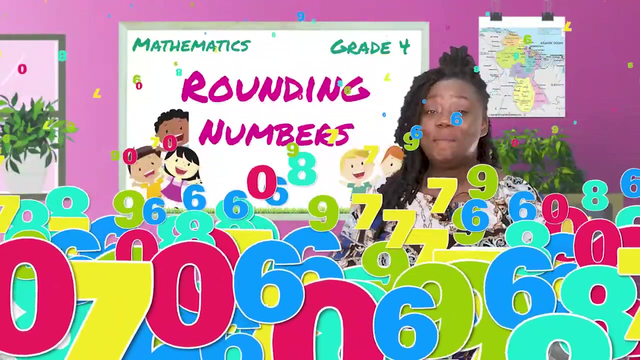 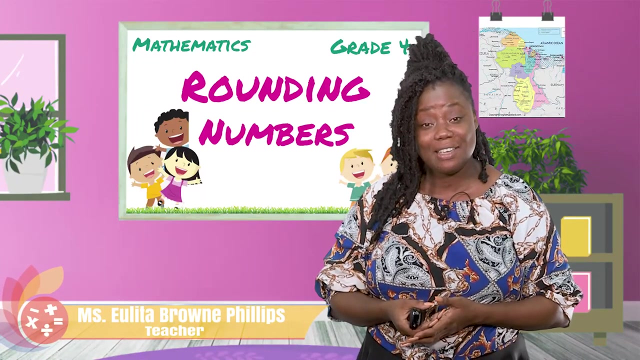 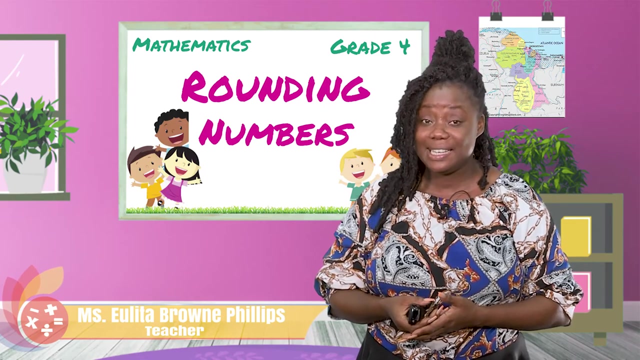 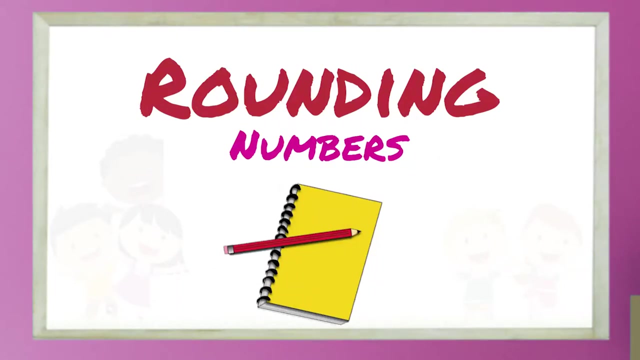 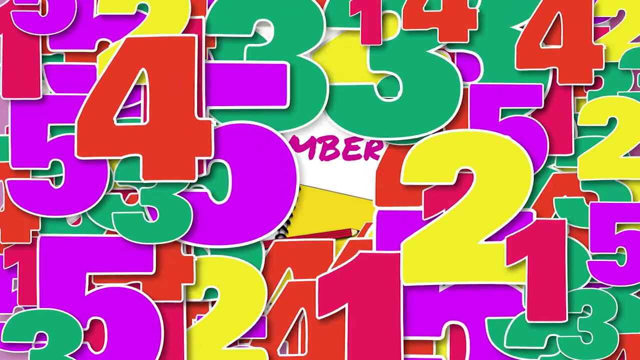 Hello, my favorite grade 4 mathematicians. How have you been? I hope that you have been staying safe and healthy. I am your mathematics teacher and in today's lesson we will be focusing on rounding numbers. So, boys and girls, grab your pens, grab your notebooks and let's take an adventure in mathematics land. Before we delve. 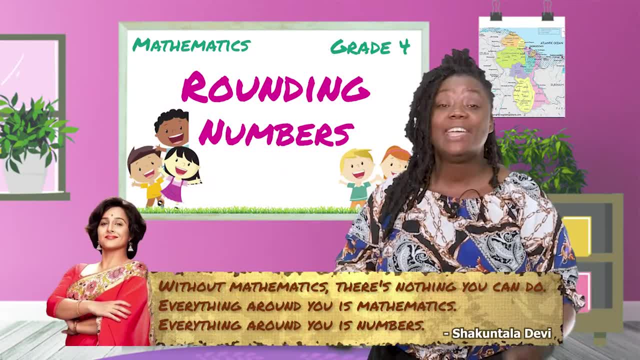 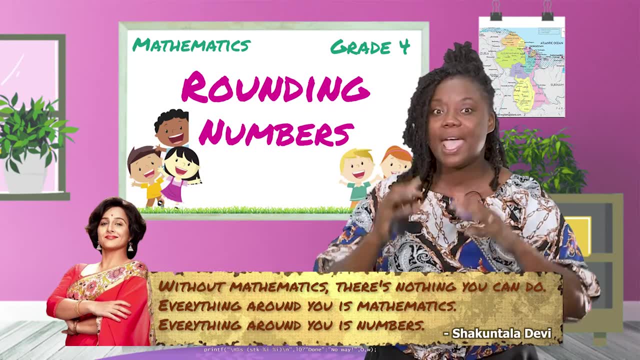 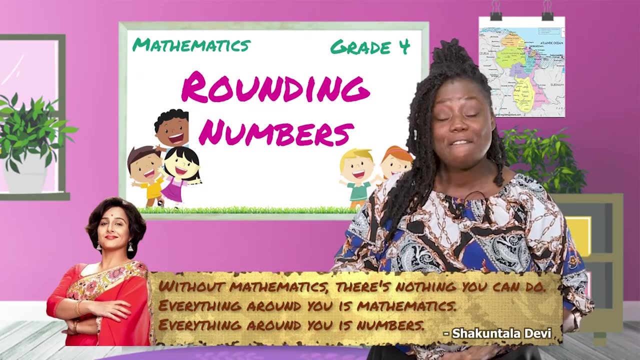 into our lesson. I want to share a quote with you. It was Shakuntala Devi who said: without mathematics, there is nothing you can do. Everything around you is mathematics, Everything around you is numbers. So, boys and girls, fasten your seatbelts. Let's take this. 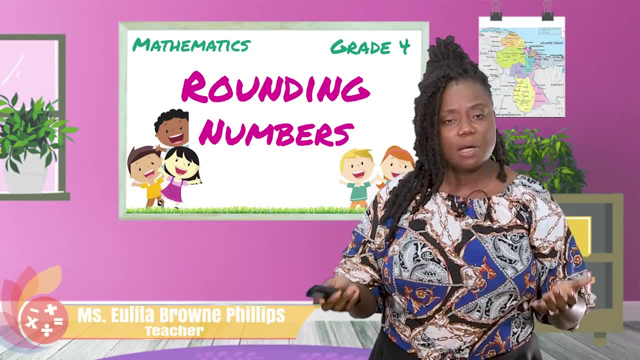 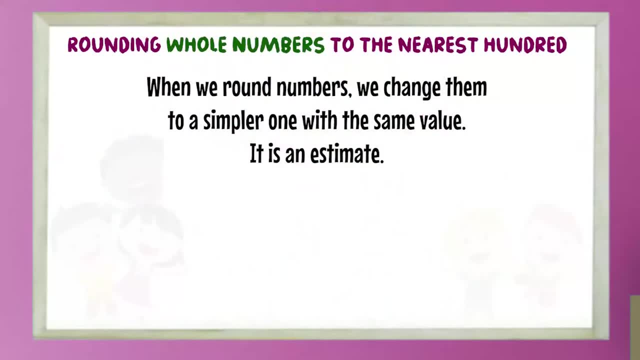 adventure in mathematics land. Our topic for today, as I told you previously, is rounding whole numbers. When we round numbers, we change them to a simpler one with the same value. It is like an estimate. Let's look at some rounding words: Estimate close enough, roughly approximate. 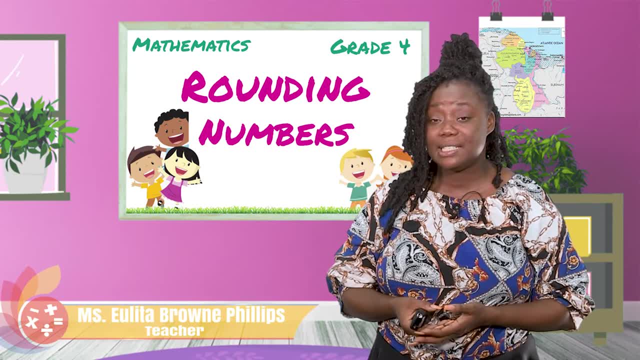 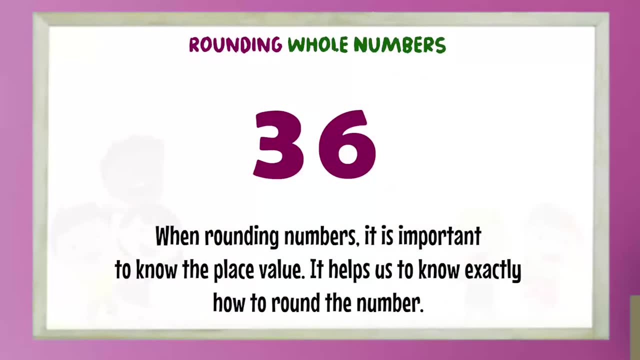 Now that we know what rounding is, let's delve in now into the meat of the matter. Let's choose a random number, 36.. When rounding numbers, it is important to know the place value. It helps us to know exactly how to round the number. I'm sure you remember what place value is. In case you don't remember, 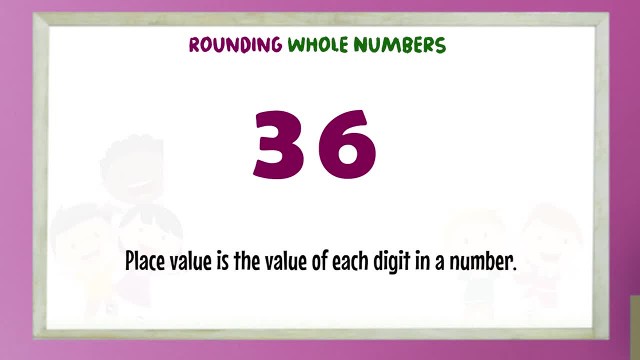 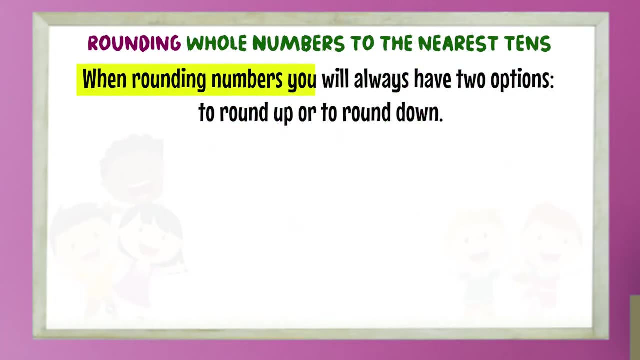 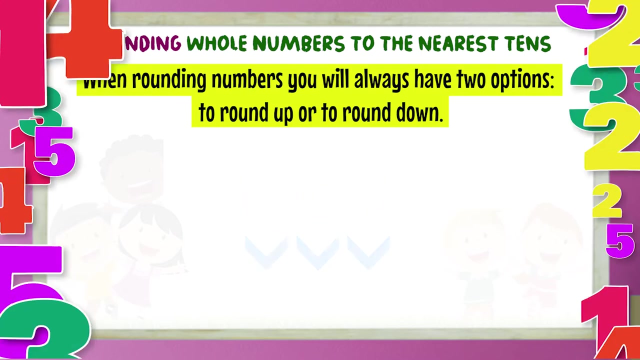 the place value of a digit is its position in the number, In the number 36,. what is the place value of the six Once? What is the place value of the six Once? What is the place value of the six? When rounding numbers, you always will have two options: Round up or round down. Examine now how to. 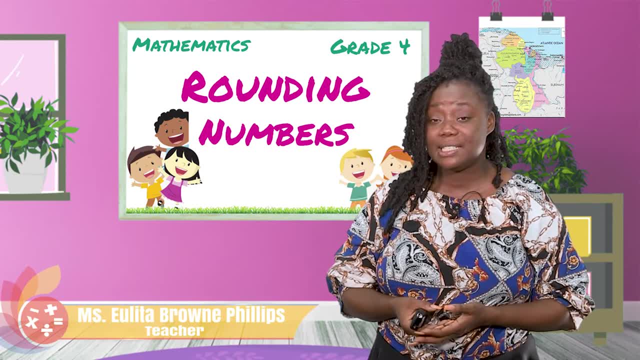 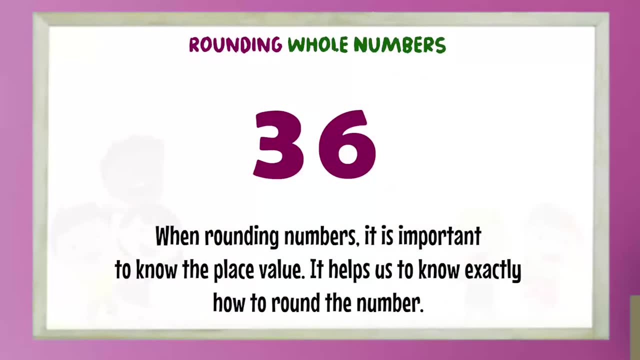 Now that we know what rounding is, let's delve in now into the meat of the matter. Let's choose a random number, 36.. When rounding numbers, it is important to know the place value. It helps us to know exactly how to round the number. I'm sure you remember what place value is. In case you don't remember, 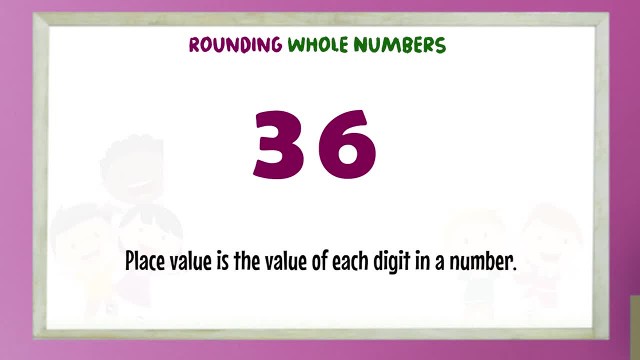 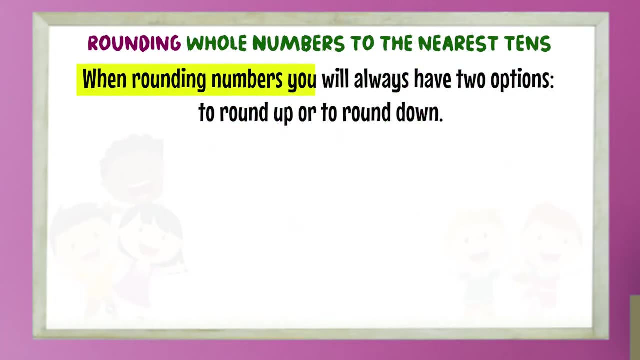 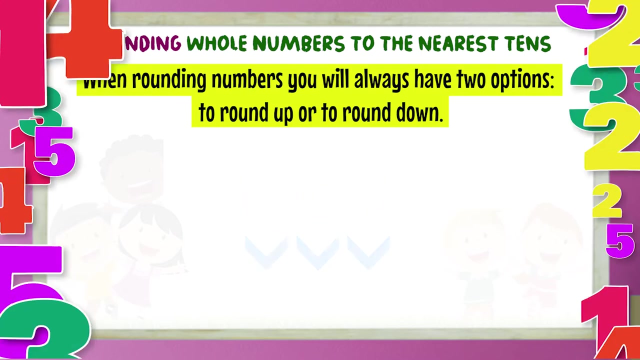 the place value of a digit is its position in the number, In the number 36,. what is the place value of the six Once? What is the place value of the six Once? What is the place value of the six? When rounding numbers, you always will have two options: Round up or round down. Examine now how to. 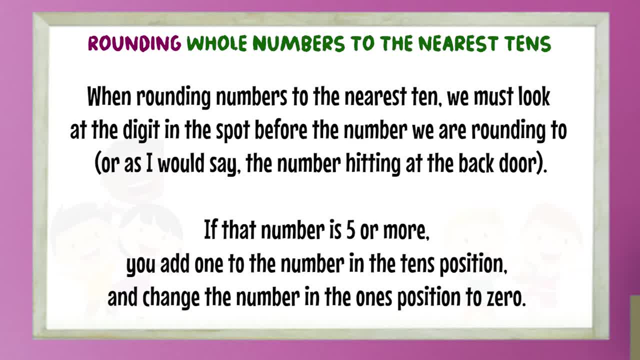 round whole numbers to the nearest 10.. When rounding numbers to the nearest 10, we must look at the digit in the spot before the number we are rounding to, Or, as I like to see, the number hitting at the back door. If that number is five or more, you add one to the number. 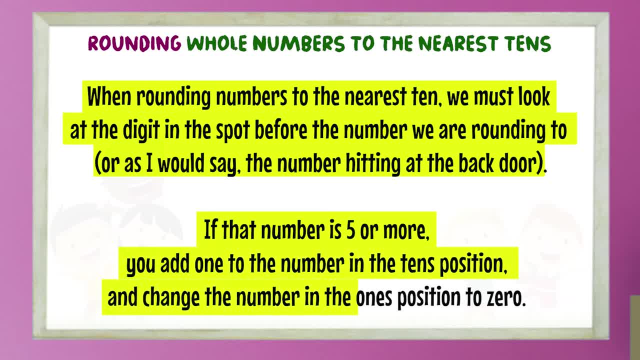 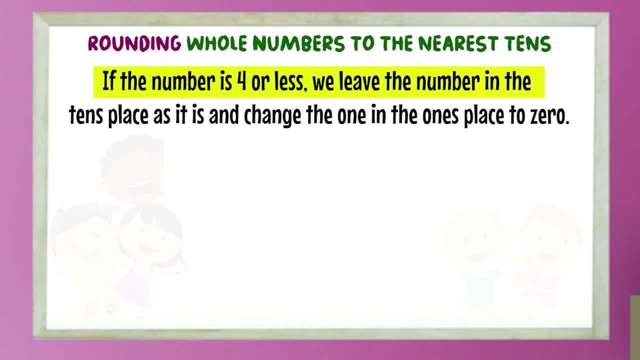 in the 10th position and change the number in the one's position to zero. If the number is four or less, we leave the number in the 10th place as it is and change the one in the one's place to zero. 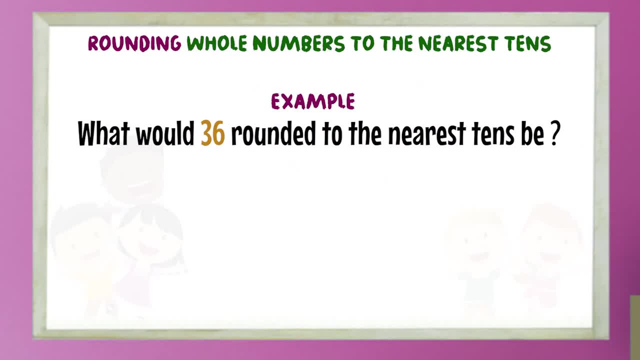 Let's look at this example: Put 36 rounded to the nearest 10's B, What number are we rounding? Hence we said that when rounding numbers, we look at the number we are rounding to first and then we look at the number that is in the place before that number. In this case, 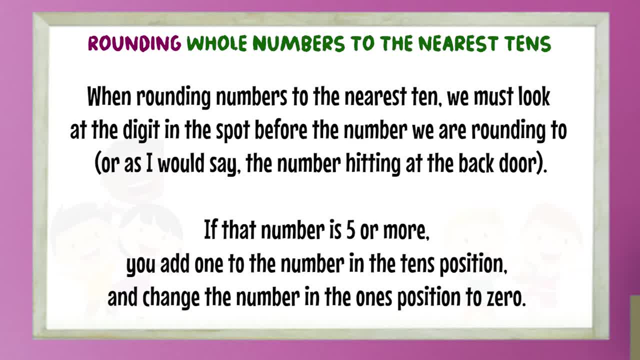 round whole numbers to the nearest 10.. When rounding numbers to the nearest 10, we must look at the digit in the spot before the number we are rounding to, Or, as I like to see, the number hitting at the back door. If that number is five or more, you add one to the number. 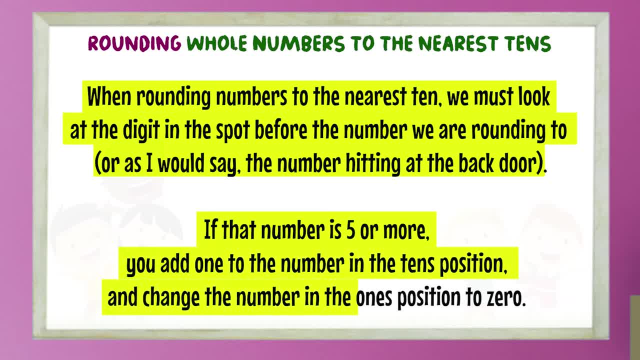 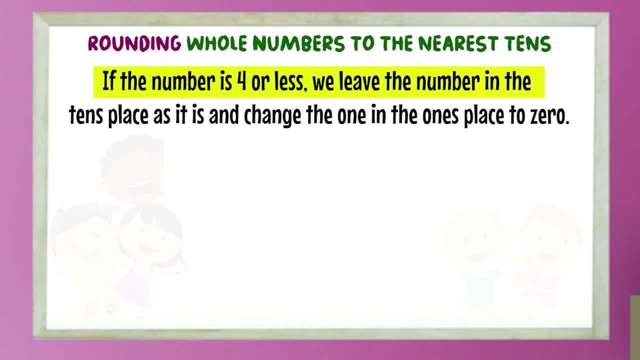 in the 10th position and change the number in the one's position to zero. If the number is four or less, we leave the number in the 10th place as it is and change the one in the one's place to zero. 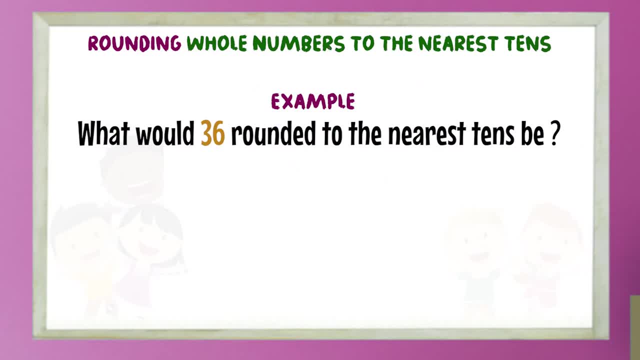 Let's look at this example: Put 36 rounded to the nearest 10's B, What number are we rounding? Hence we said that when rounding numbers, we look at the number we are rounding to first and then we look at the number that is in the place before that number. In this case, 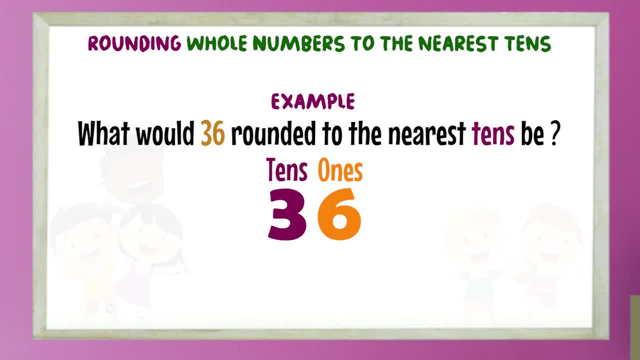 six is in the place before that number. Is six, more than five or less than five? Six is more than five. Since six is more than five, we add one to the number in the 10's column and change the number in the one's column to zero. 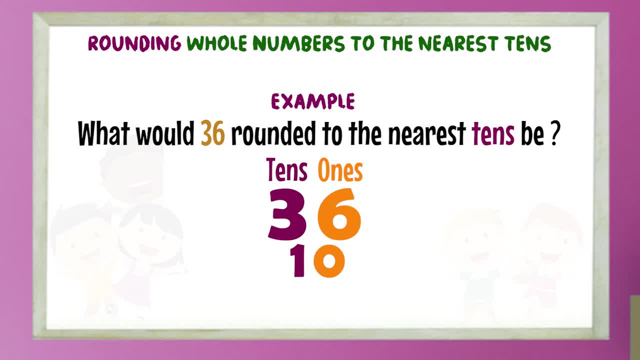 So three plus one will give us four, and the six is changed to a zero. So 36 rounded to the nearest 10's is 40.. Let's look at another example. What is 454 rounded to the nearest 10?? 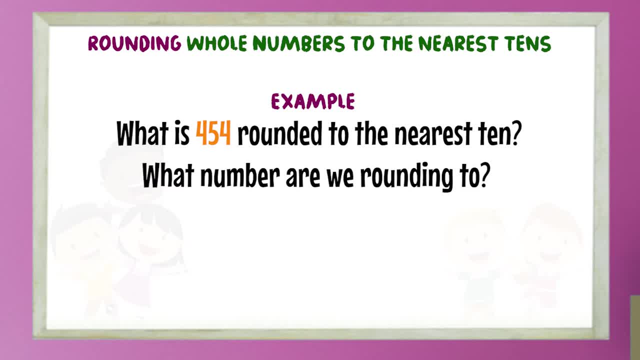 Question 5: What number are we rounding to? A B C, F A B C, F B, A B C, F A B C, F, B, A B C. 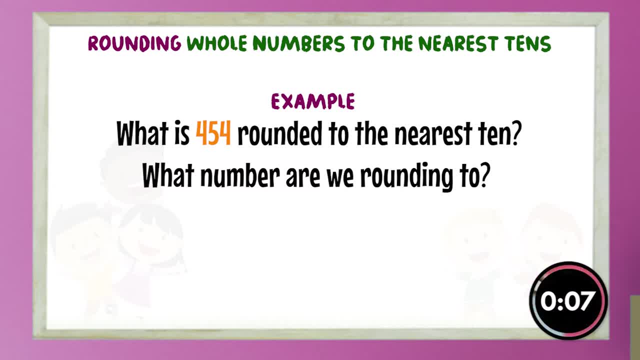 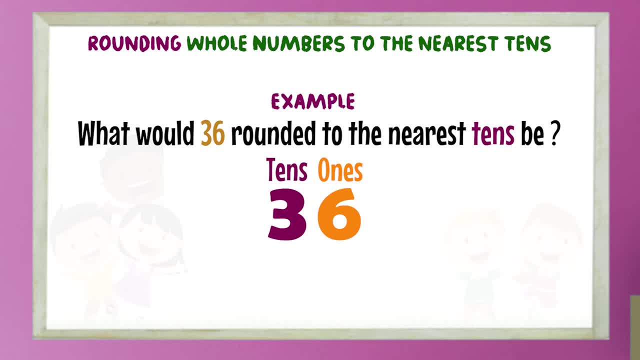 six is in the place before that number. Is six more than five or less than five? Six is more than five. What is the place value of the six? Since six is more than five, we add 1 to the number in the tens column and change the number in the ones column to 0.. 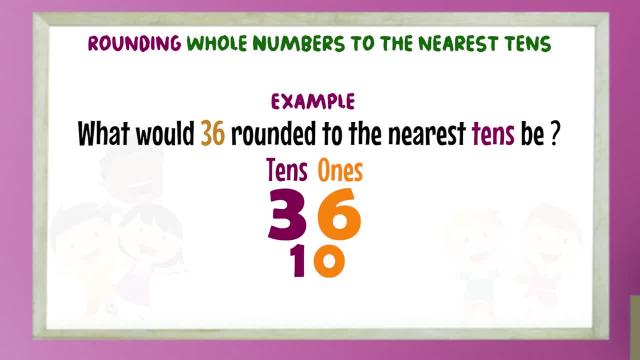 So 3 plus 1 will give us 4, and the 6 is changed to a 0. So 36 rounded to the nearest tens is 40.. Let's look at another example. What is 454 rounded to the nearest 10?? 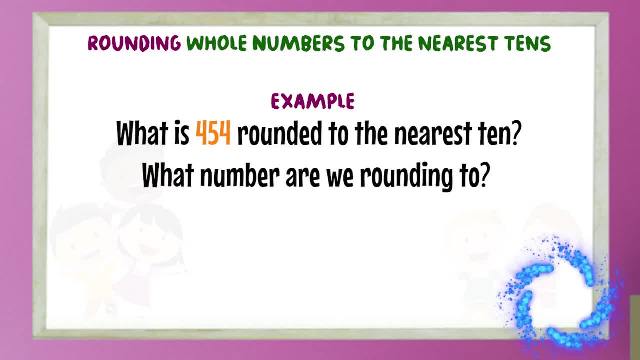 What number are we rounding to? We are rounding the number to the nearest 10.. What is the number in the tens place in that number? The number in the tens place in that number is 5.. So, now that we would have identified our number that we are rounding, 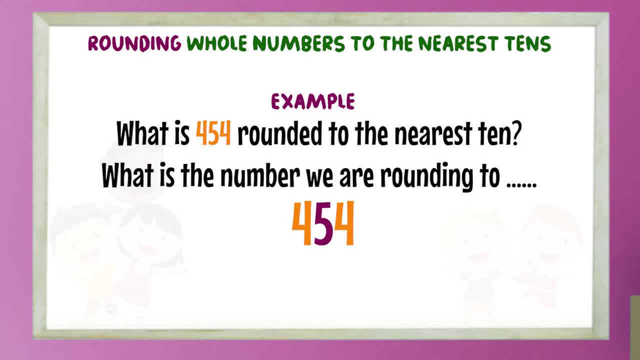 let's identify the number in the position before that number or the number hitting on the back door. That number is 4.. Is 4 more than 5 or is it less than 5?? 4 is less than 5.. We said if the number in the ones place is less than 5,. 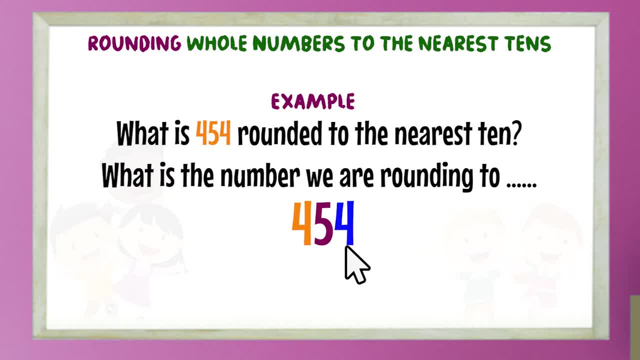 we write back the number in the tens place as is and change the number in the ones place to 0. So we will write back our 4,, we will write back our 5, and we will change the 4 to 0.. 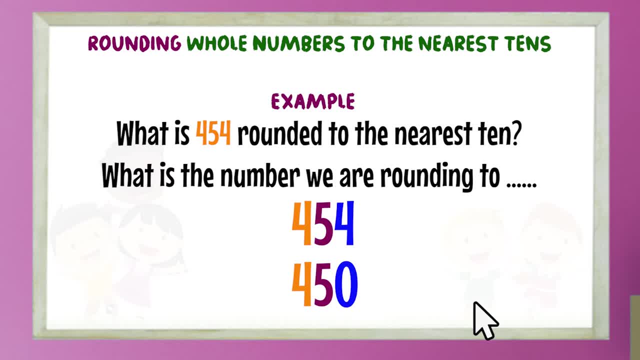 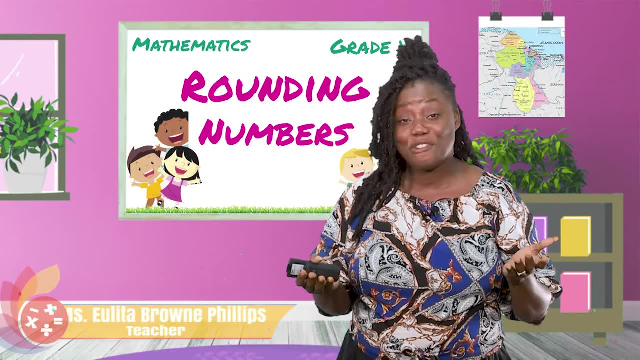 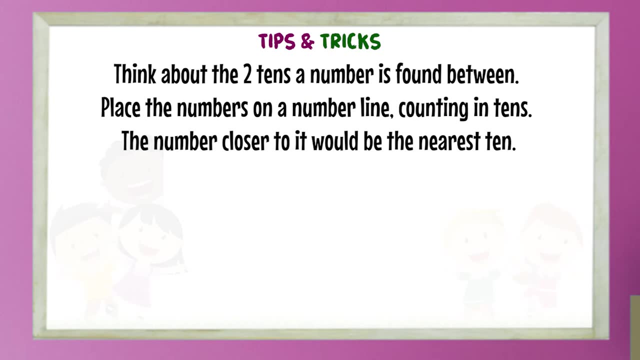 So 454, rounded to the nearest 10. Is 450.. Boys and girls, it is now time for our tips and tricks segment. Now, this is a tip and a trick for when you are rounding numbers to the nearest 10.. Listen carefully. 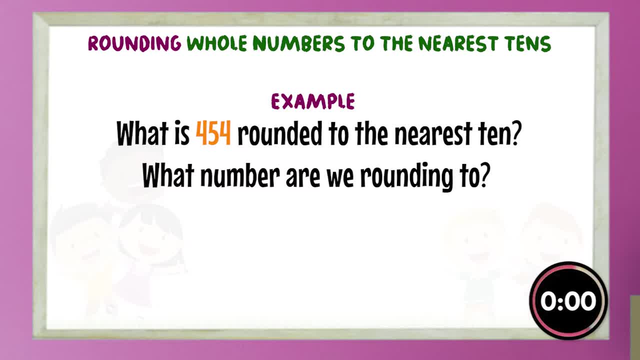 B B C F, B, B C, F, B, B C F. We are rounding the number to the nearest 10's, B. next here in .5: After 2, that'm going to be 5 points, Army. I will count it by 3. last number: total .5AB. 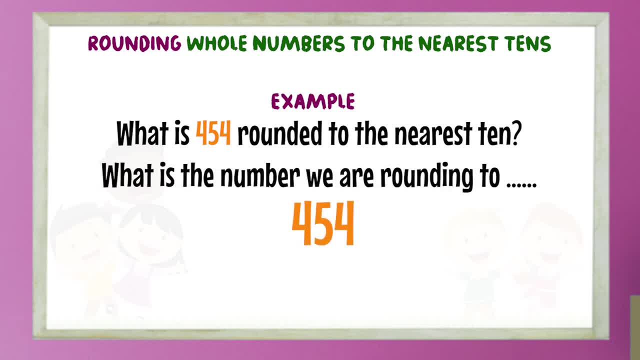 number to the nearest 10.. What is the number in the 10th place in that number? The number in the 10th place in that number is 5.. So, now that we would have identified our number that we are rounding, let's identify the number in the position before that number or the number hitting on the. 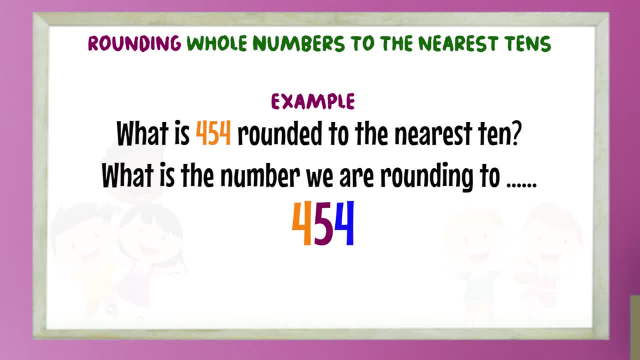 back door. That number is 4.. Is 4 more than 5 or is it less than 5?? 4 is less than 5.. We said if the number in the 1st place is less than 5, we write back the number in the 10th place as is. 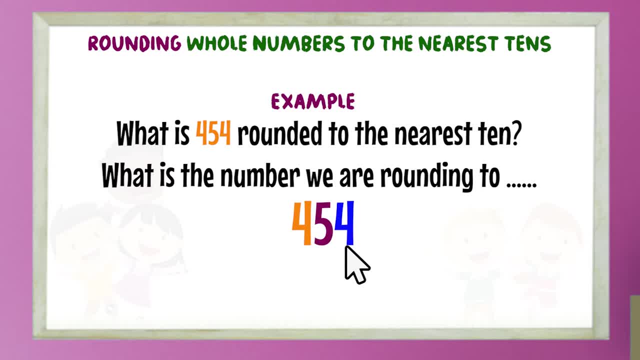 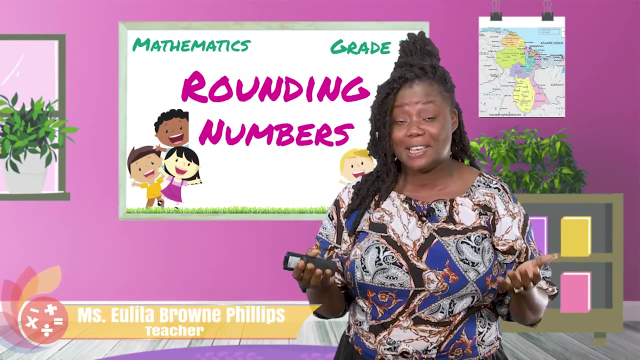 and change the number in the 1st place to 0.. So we will write back our 4, we will write back our 5 and we will change the 4 to 0. So 454 rounded to the nearest 10 is 450.. Boys and girls, it is now time for our tips and tricks segment. Now this: 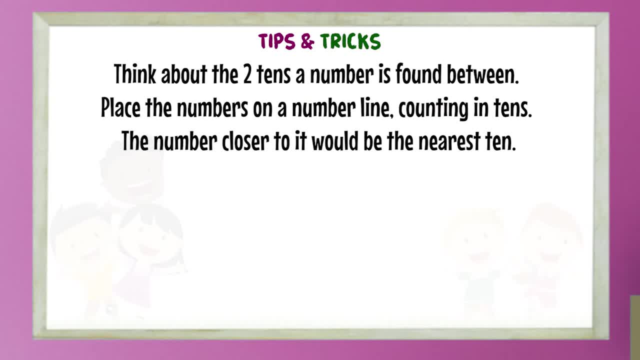 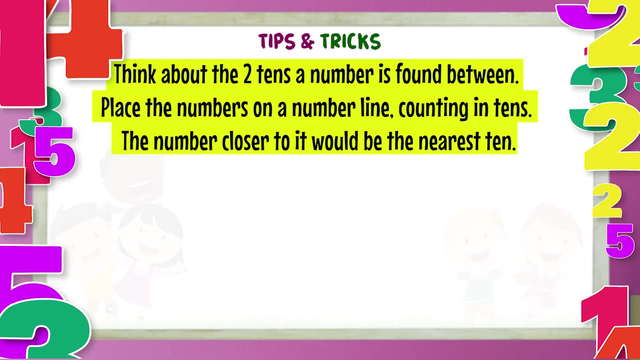 is a tip and a trick for when you are rounding numbers to the nearest 10.. Listen carefully Now you think about the two 10's. a number is found between You can't place them on a number line counting in 10's. The number closer to it would be the nearest 10.. Let's quickly look at. 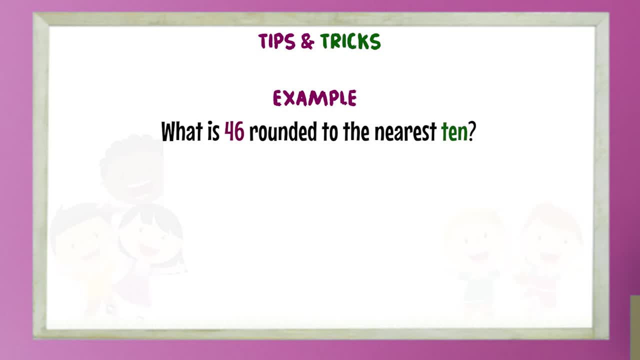 this example: What is 46 rounded to the nearest 10?? So let's get our number line up there, counting in 10's. So we know that a number line always starts from 40. So how do we know 50 is? greater than 50?? I'm going to show you guys what a number line is. Let's see. If you go to list revenue And fields, andungen HYBR, пон breaker and units, you'll find that this column is meeting 10, and if you recognize 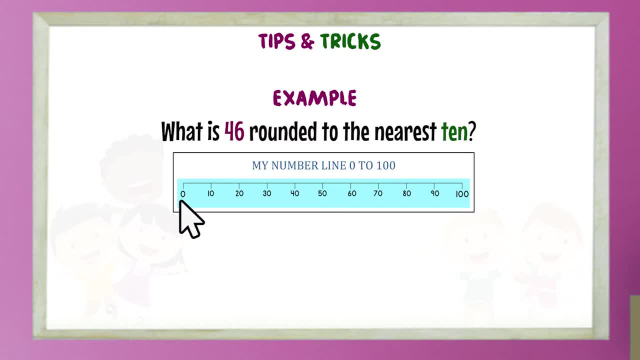 always starts with zero. So we have our zero: 10, 20,, 30,, 40,, 50,, 60.. Let's stop at 60.. Where do you think 46 is found on this number line? Which two numbers 46 falls between? 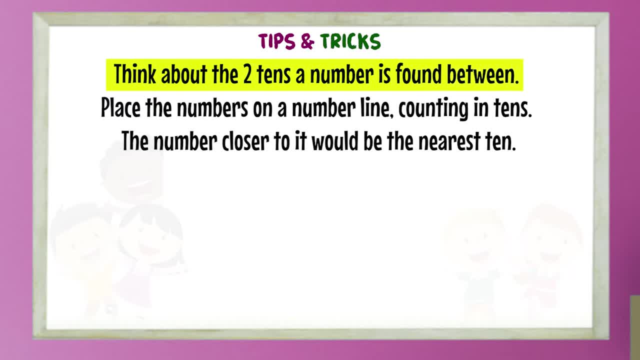 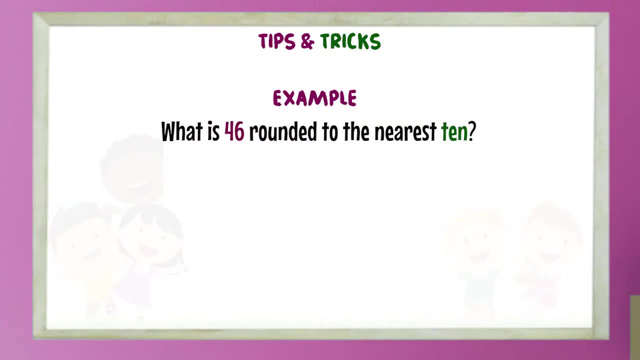 Now you think about the two tens. a number is found between You can't place them on a number line. counting in tens, The number closer to it would be the nearest 10.. Let's quickly look at this example. What is 46 rounded to the nearest 10?? 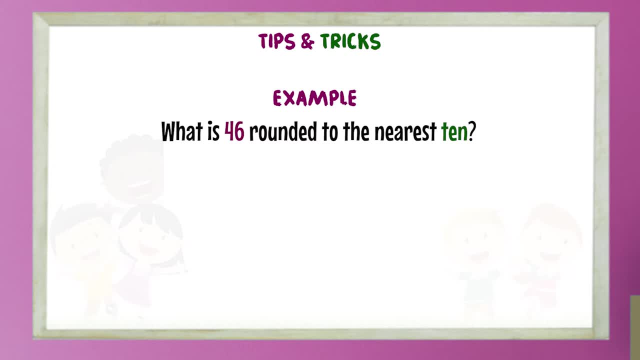 So let's get our number line up there, counting in tens, So we know that a number line always starts with 0. So we have our 0, 10,, 20,, 30,, 40,, 50,, 60.. 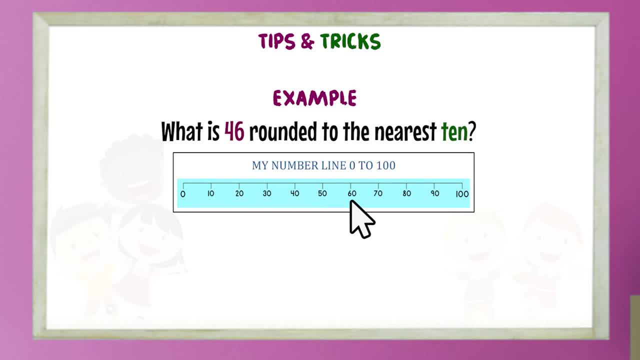 Let's stop at 60.. So we know we are rounding numbers. at least 20, Join us. We have worked all days till now and you are looking to remember 46. So you should be asking yourself a question: What is 46,? where do you think 46 is found on this number line? 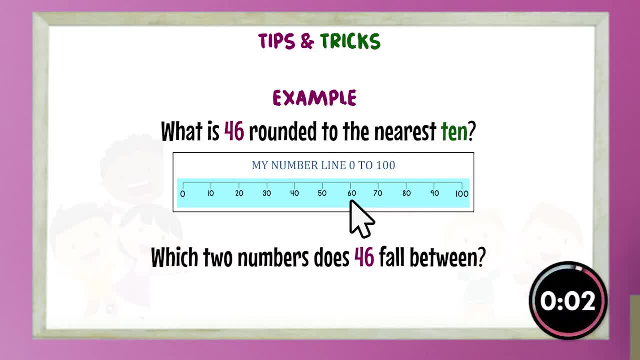 Which two numbers 46 falls between? Answer me. Did you say 40 and 50?? Yes, you are absolutely correct. 46 falls between 40 and 50. Now which number is it closer to? Is 46 closer to 40, or is 46 closer to 50?? 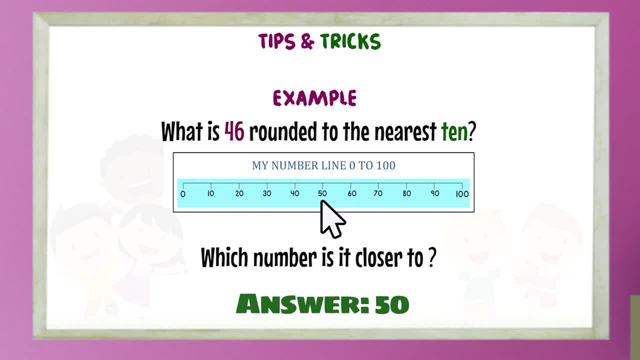 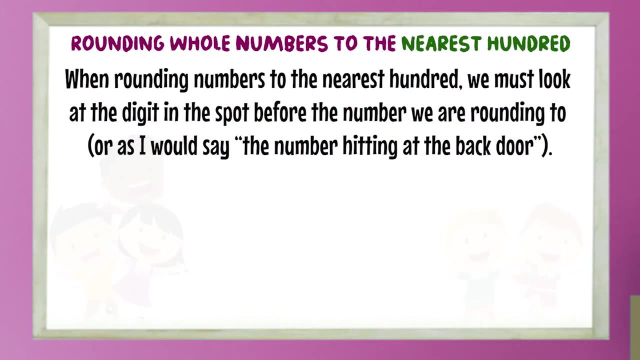 Did you say 50?? Well then, you are absolutely correct. 46 is closest to 50.. So 46 rounded to the nearest 10 is 50.. Boys and girls, let's move on to rounding whole numbers to the nearest 100. 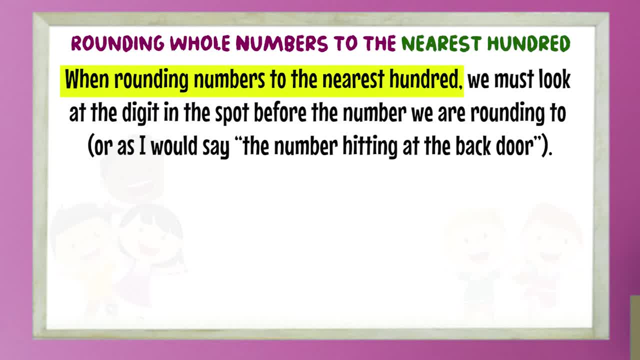 When rounding numbers to the nearest 100, we must look at the digit in the spot before the number we are rounding. Rounding 2, or, as I would say, the number hitting on the back door, In other words, boys and girls. when rounding numbers to the nearest 100, we look at the number in the 10's place. 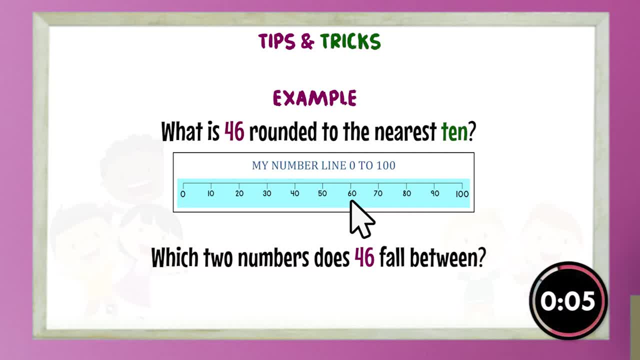 Good, Did you say 40 and 50?? Yes, you are absolutely correct. 46 falls between 40 and 50. Now, which number is it closer to? Is 46 closer to 40, or is 40 closer to 60?? 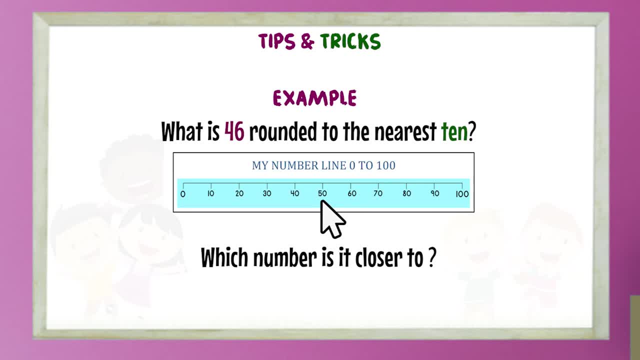 Is 46 closer to 40, or is 40 closer to 60?? Is 46 closer to 40 or is 40 close to 60?? 46 closer to 50. Did you say 50?? Well then, you are absolutely correct: 46 is closest. 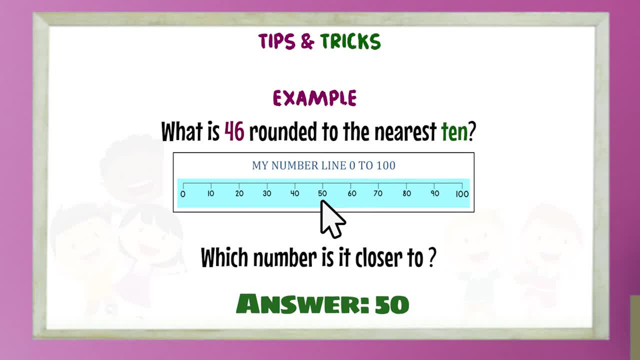 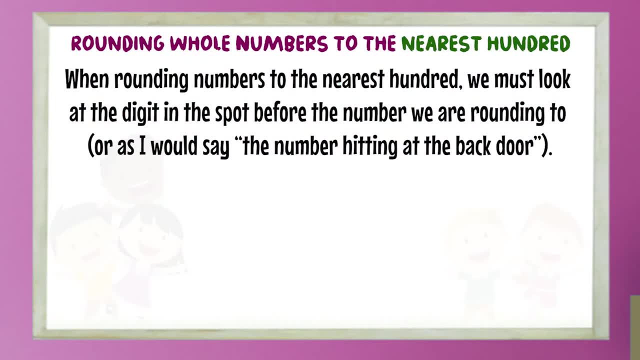 to 50. So 46 rounded to the nearest 10 is 50.. Boys and girls, let's move on to rounding whole numbers to the nearest 100.. When rounding numbers to the nearest 100, we must look at the digit in the spot before the number we are rounding to, or, as I would say, the number. 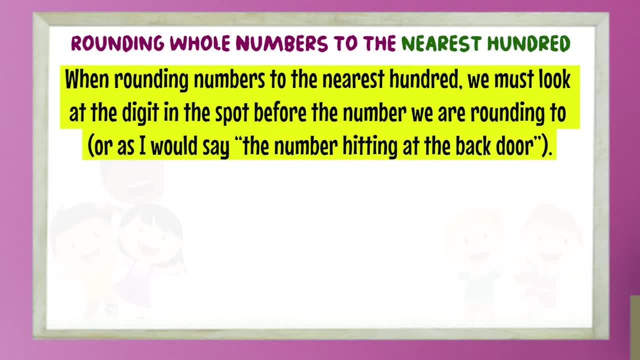 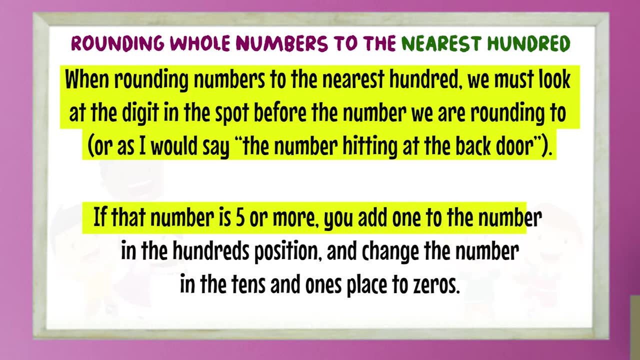 hitting on the back door, In other words, boys and girls. when rounding numbers to the nearest 100, we look at the number in the tens place. If the number is 5 or more, you add 1 to the number in the hundreds place and you change the number in the tens place. 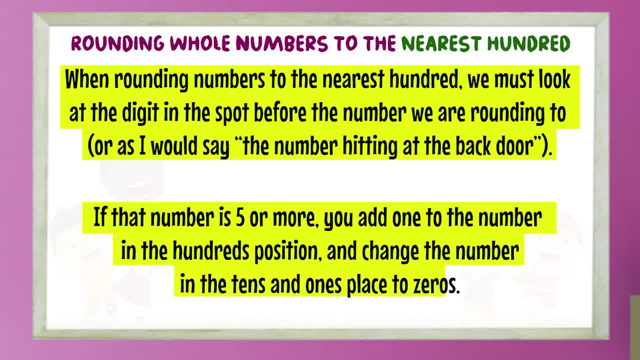 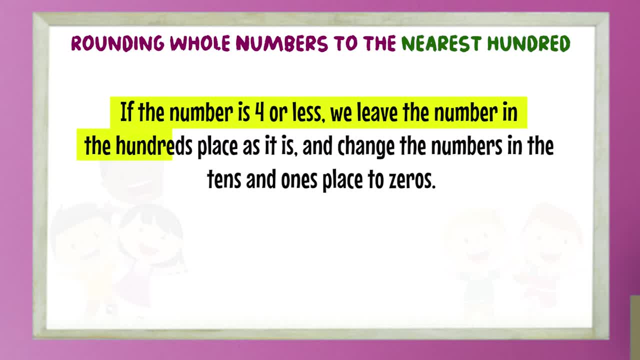 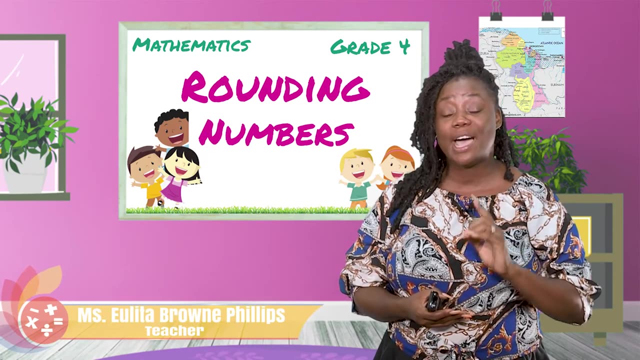 and the ones place to zeros. If the number is less, we leave the number in the hundreds place as is and we change the numbers in the tens and the ones place to zero. So when rounding numbers to the nearest 100, you look at the number in the tens position. Let's 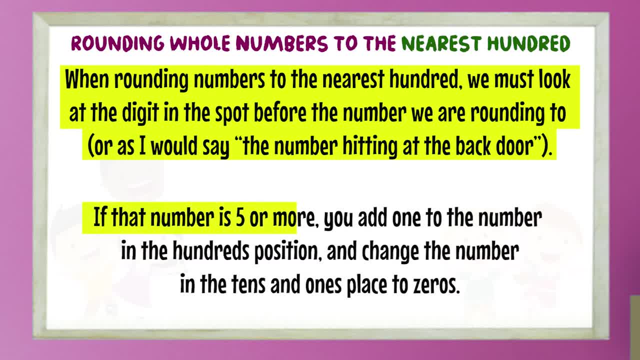 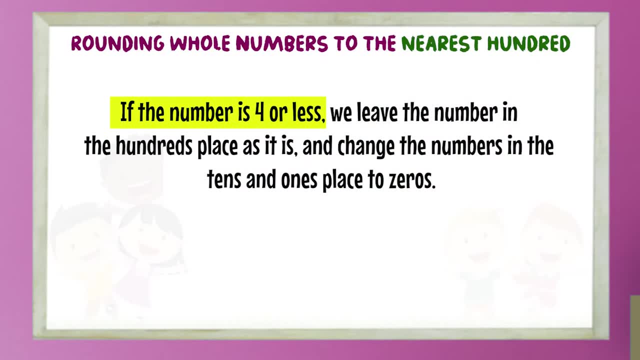 If the number is 5 or more, you add 1 to the number in the 100's place and you change the number in the 10's and the 1's place to 0.. If the number is less, we leave the number in the 100's place as is. 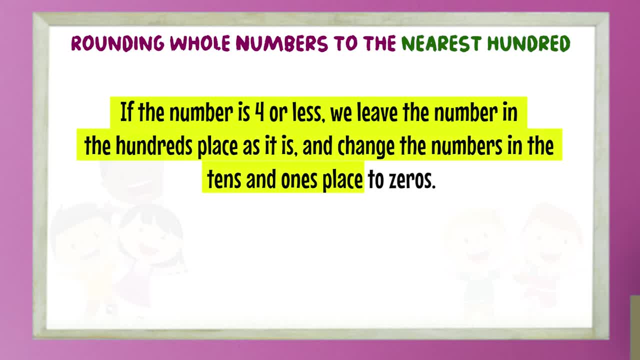 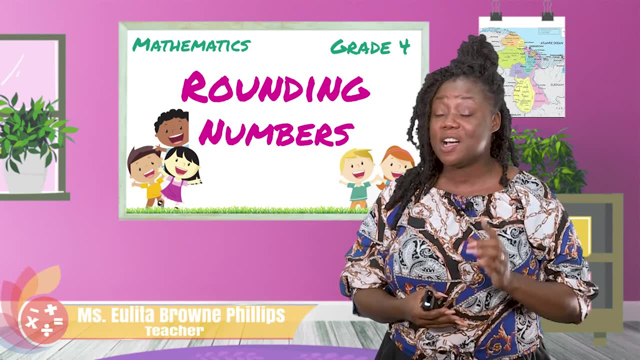 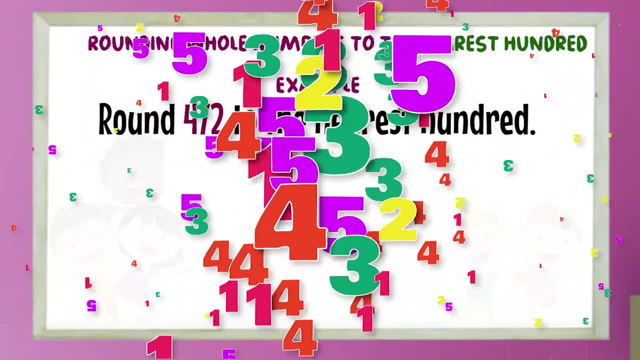 and we change the numbers in the 10's and the 1's place to 0. So when rounding numbers to the nearest 100, you look at the number in the 10's position. Let's quickly look at an example. 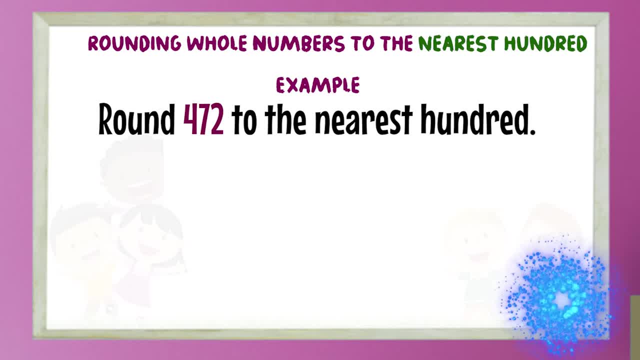 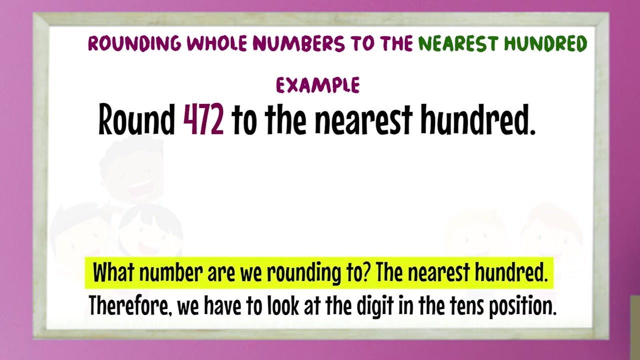 Round 472 to the nearest 100.. Round 474 to the nearest 100.. What number are we rounding to? Round 474 to the nearest 100.. Round 474 to the nearest 100.. Therefore, we have to look at the digit in the tens position. 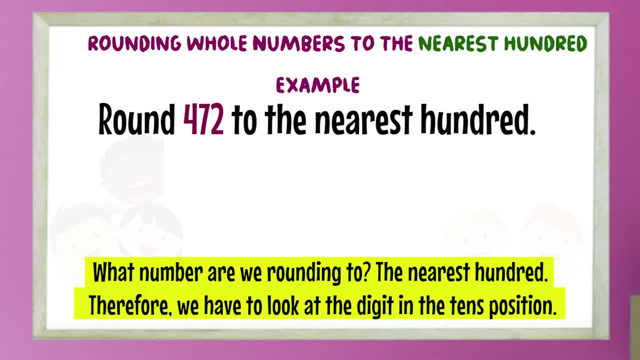 What is the number in the tens position? Seven Is seven more than five or is it less than five? boys and girls. Seven is more than five. We said if the number in the tens place is seven or more, we add one to the number in the hundreds place and we change the numbers in the tens and the ones place to zero. 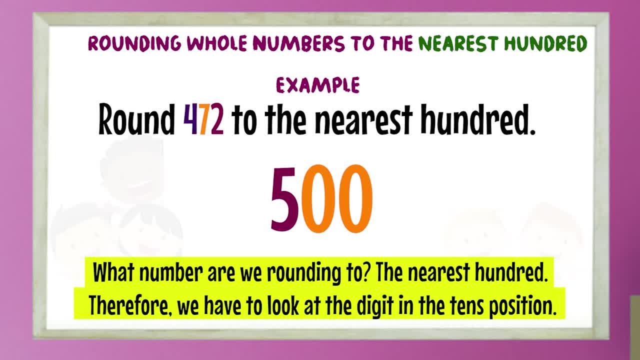 What is the number in the hundreds place Four. When one is added to that four, it becomes five. The rule said we change the numbers in the ones Ones and the tens place to zero. Therefore, 472 rounded to the nearest hundred is 500.. 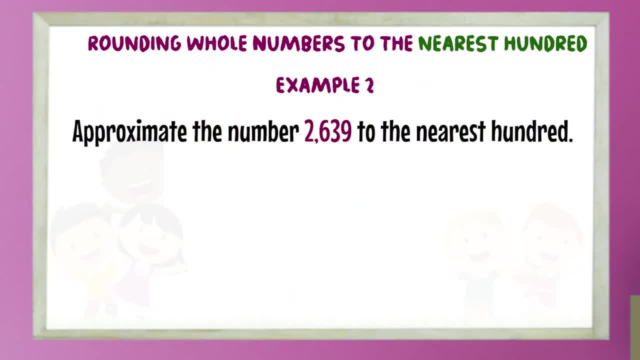 Let's look at example two. Approximate the number 2,639 to the nearest hundred. Boys and girls. did you notice I used a different word instead of rounding: approximate. It means the same thing. All you're simply asked to do is to round 2,639 to the nearest hundred. 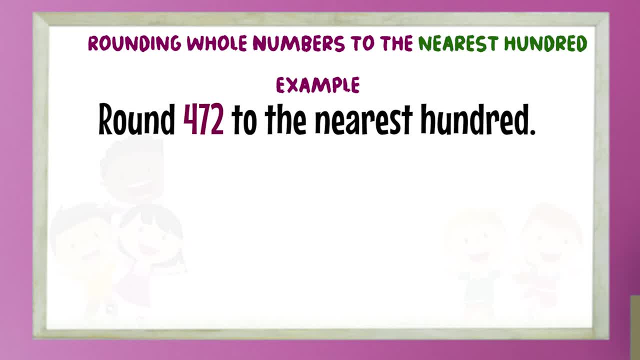 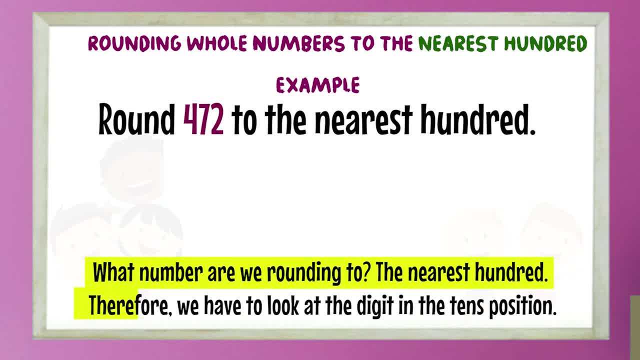 the nearest 100.. Therefore we have to look at the digit in the tens position. What is the number in the tens position? Seven, Is seven more than five or is it less than five? boys and girls? Seven is more than five, We said if the number in the tens place is seven or more. 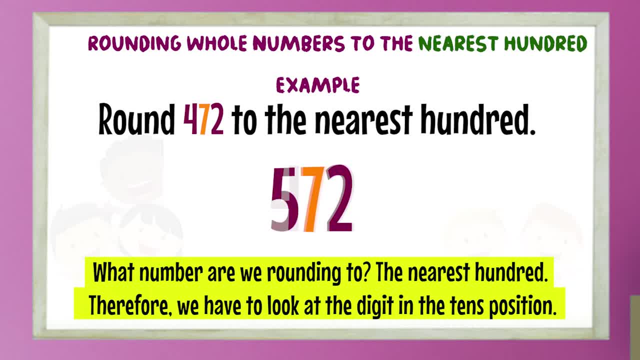 we add one to the number in the hundreds place and we change the numbers in the tens and the ones place to zero. What is the number in the hundreds place Four? When one is added to that four, it becomes five. The rule said: we change the numbers in the ones and the tens place to zero. Therefore, 472 rounded. 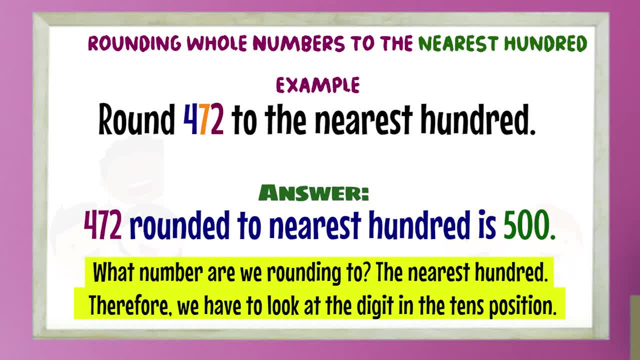 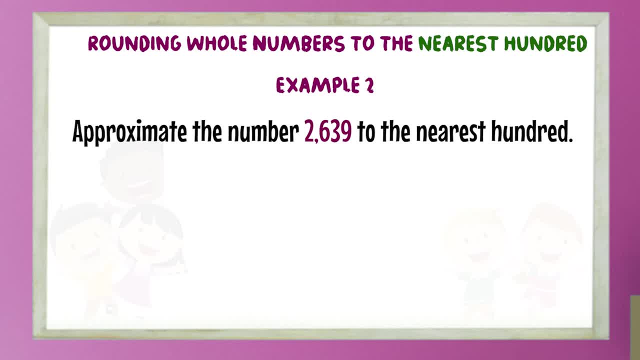 to the nearest 100 is 500.. Let's look at example two. Approximate the number 2,639 to the nearest hundred Boys and girls. did you notice I used a different word instead of rounding Approximate? It means the same thing. All you're simply asked to do is to round 2,639. 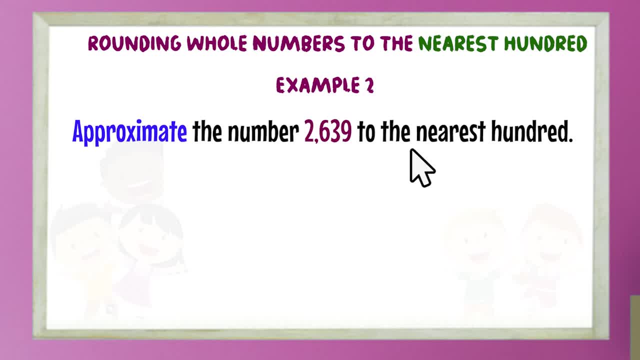 by 2,639 to the nearest hundred. So let's identify our digit that we are rounding to. We are rounding to the nearest hundred. The number in the hundreds place is six. Let's identify the digit to the right of that number, or, as I would say, the number that is hitting. 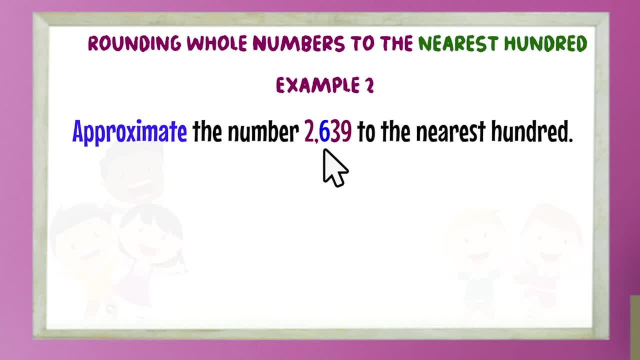 that number's back door. The number red is room number. The number blue is the number Dreamy number. The number blue is the number sp inspireent. The would be B or red. The word Dreamy is a combination. All of them would be B or red. It would. 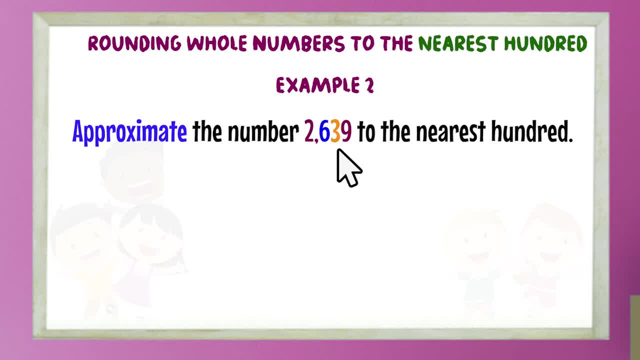 is 3, the number in the tens position is 3 greater than 5 or is it less than 5?? We know that 3 is less than 5.. We establish when the number in the tens place is less than 5,. 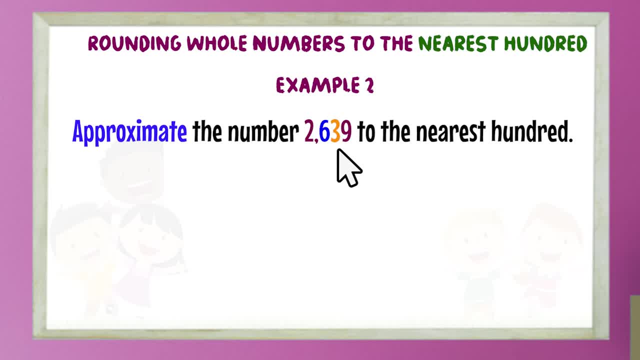 we leave the number in the hundreds place as is and we change the numbers in the tens and the ones place to zero. So we write back our 2, we write back our 6 and we add two zeros, since we are rounding to the nearest hundred. Boys and girls, it is time for you to put into 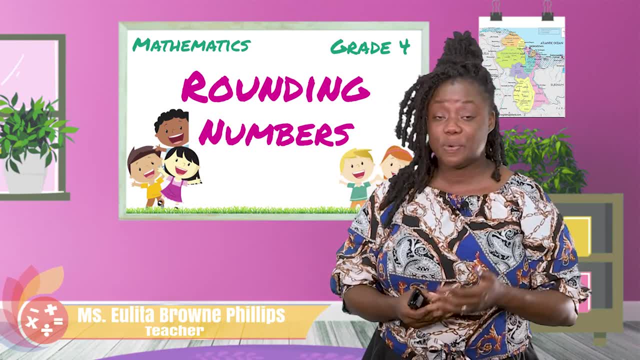 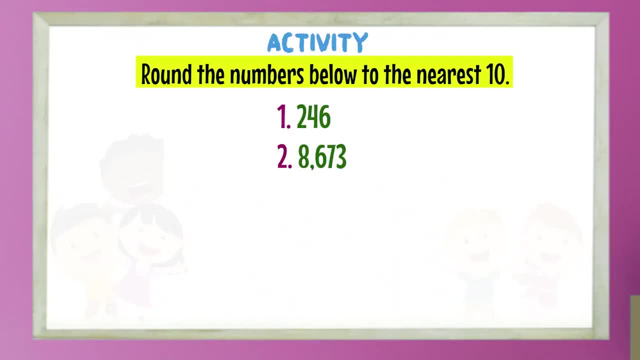 practice what you would have learned. So here is an activity. Round the numbers below to the nearest ten. Number 1, 246.. Number 2, 8,673.. Let's see what you have. You should be finished by now. 246. 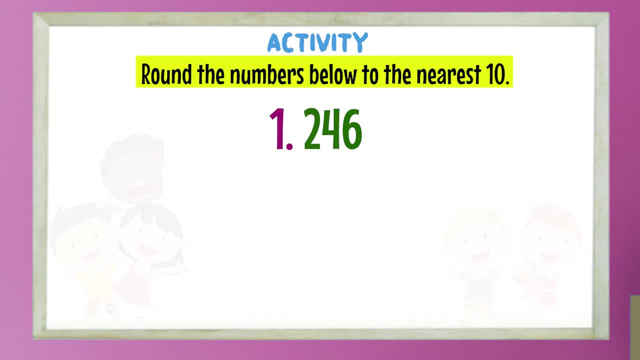 We are rounding to the nearest ten, so we look at the number in the ones place. What number is in the ones place? boys and girls, 6. Is 6 more than 5 or is it less than 5?? 6 is more than 5 and we learned that once the number in the ones place is more than 5,. 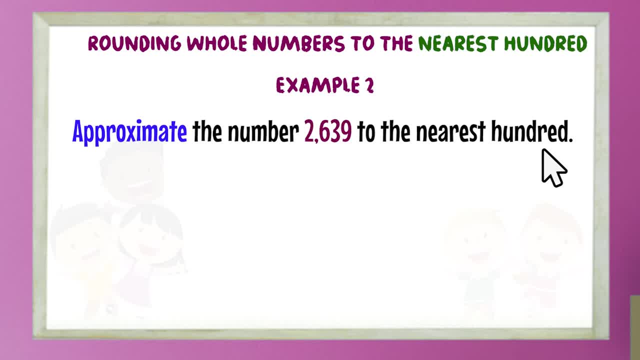 So let's identify our digit that we are rounding to. We are rounding to the nearest hundred. The number in the hundreds place is six. Let's identify the digit to the right of that number, Or, as I would say, the number that is right. 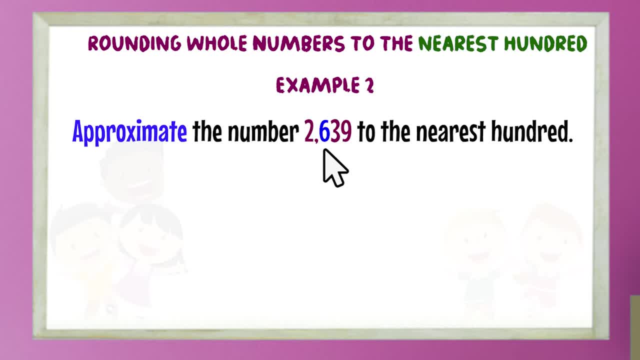 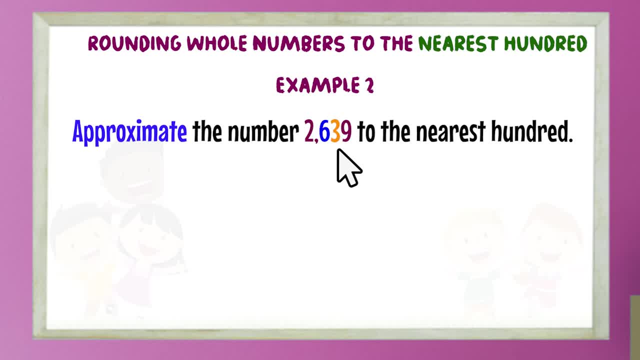 We establish: when the number in the tens place is less than five, we leave the number in the hundreds place as is and we change the numbers in the tens and the ones place to zero. So we write back our two, we write back our six and we add two zeros, since we are rounding to. 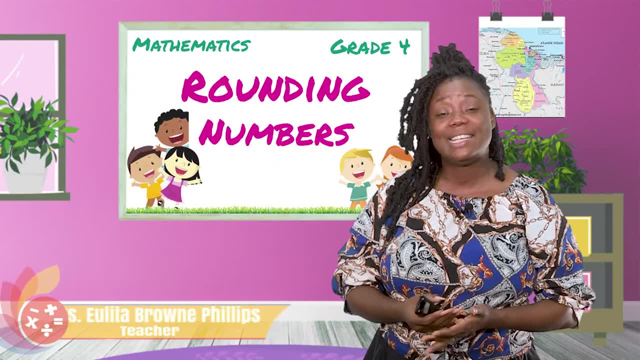 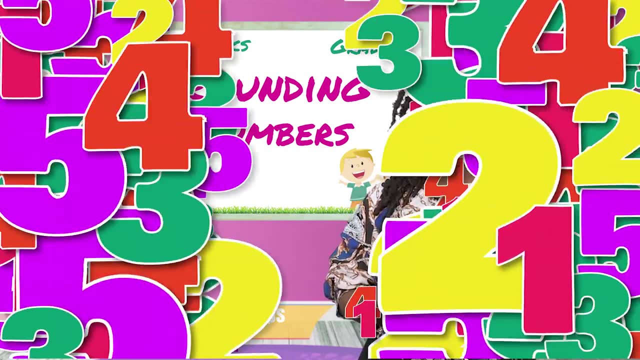 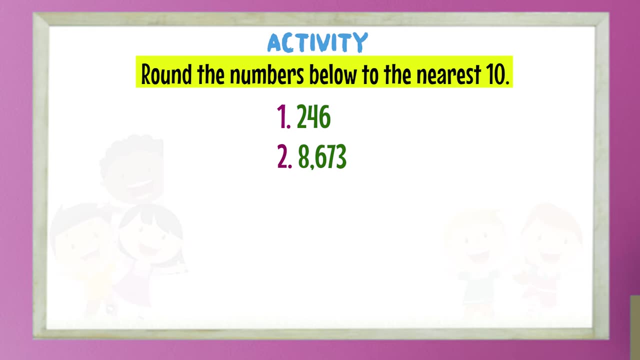 the nearest hundred Boys and girls. it is time for you to put into practice what you would have learned. So here is an activity: Round the numbers below to the nearest ten. Number one: two hundred forty-six. Number two: eight thousand six hundred. 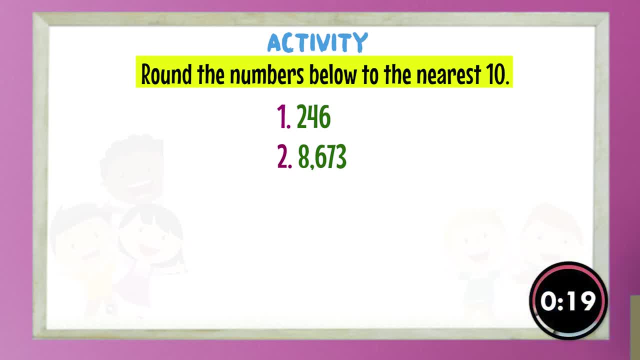 seventy-three. Let's see what you have. You should be finished by now. Two hundred forty-six: We are rounding to the nearest ten. So we look at the number in the ones place. What number is in the ones place, boys and girls? Six Is six more than five or is it less than five? Six is more than five. 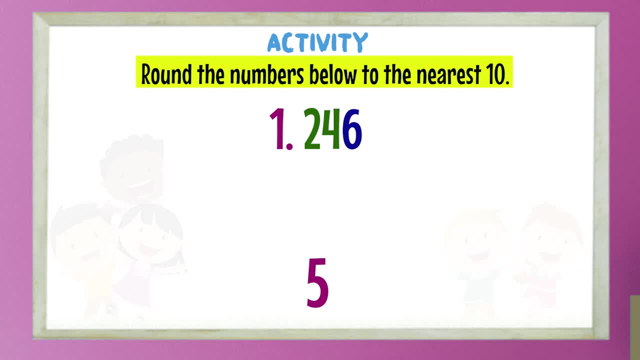 And we learned that once the number in the ones place is more than five, we add one to the number in the tens place and we change the number in the ones place to zero, because we are rounding to the nearest ten. Therefore, two hundred forty-six rounded to the nearest ten is two hundred fifty. 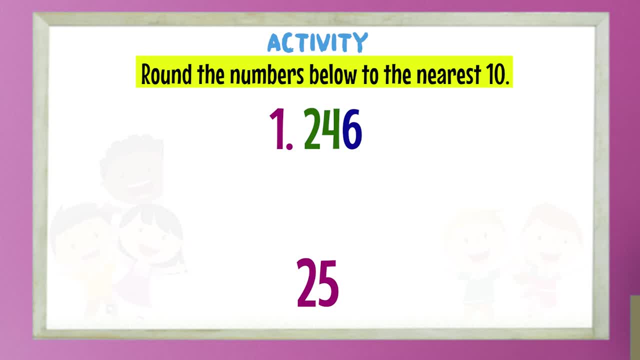 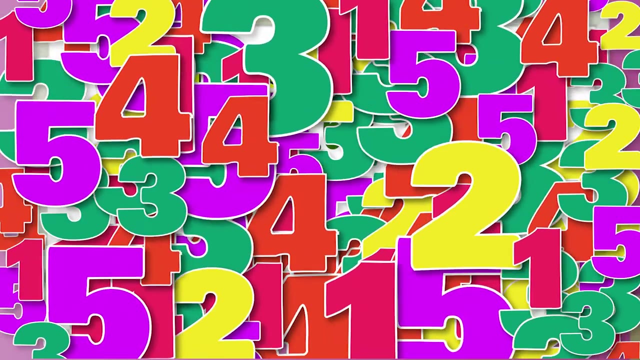 we add 1 to the number in the tens place and we change the number in the ones place to zero, because we are rounding to the nearest ten. Therefore, 246 rounded to the nearest ten is 250.. Let's look at the other one: 8,673 rounded to the nearest ten. 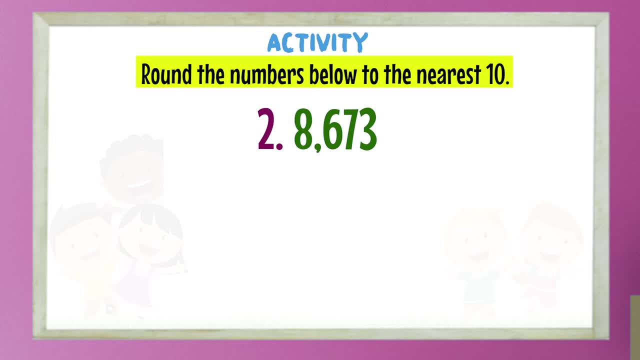 Let's identify the number we are rounding to the nearest: 10. The number in the tens place is 7.. Which number is to the right of that number, or which number is hitting the back door of that number? 3. Is 3 more than 5 or is it less than 5?? 3 is less than 5.. 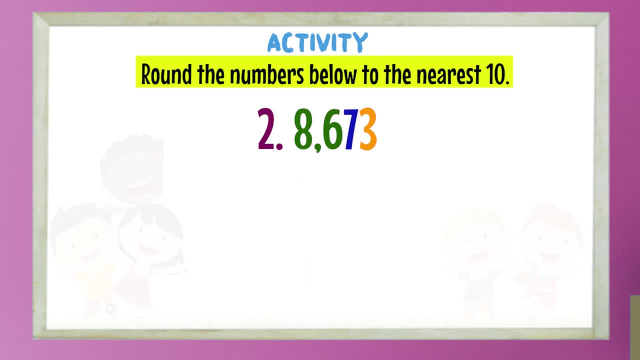 than five. We learnt that if the number in the ones place is less than five, we rewrite the number as is and change the number in the ones place to zero. So we write back our eight, our six, our seven and we change the three to zero. Eight thousand six hundred. 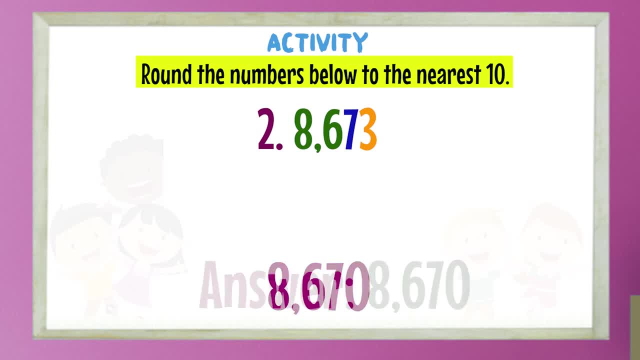 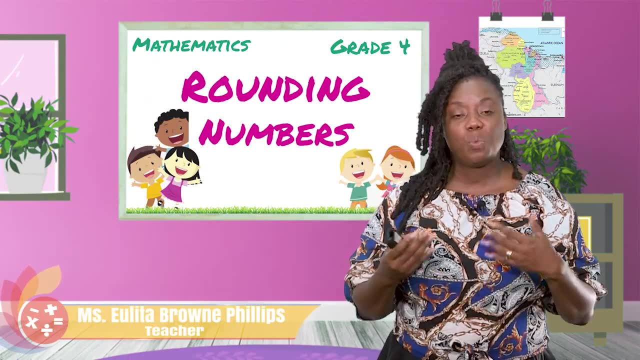 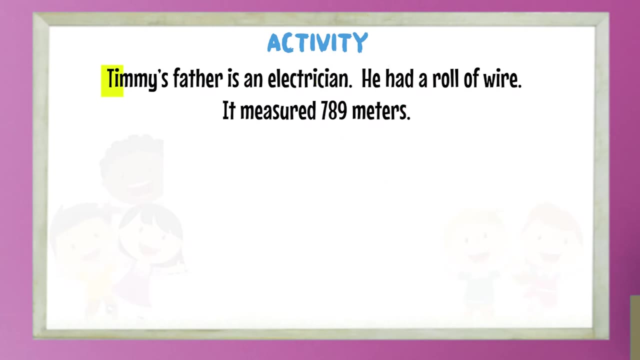 seventy-three rounded to the nearest ten is eight thousand six hundred seventy Boys and girls. there is one other activity I want you to do, but this is in the form of a problem. Timmy's father is an electrician. He had a roll of wire. It measured seven hundred. 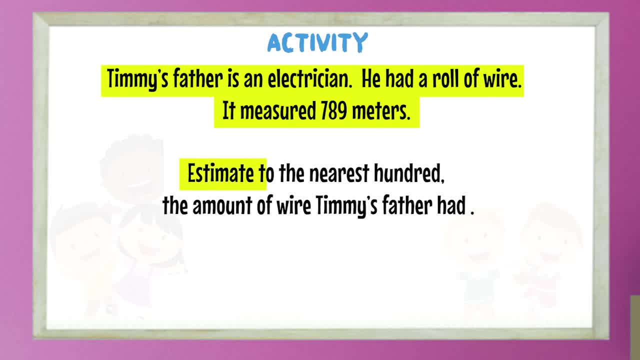 eighty-nine meters. Estimate to the nearest hundred The amount of wire Timmy's father had Boys and girls. did you notice I used another rounding word: Estimate. All it simply means is that you have to round seven hundred eighty-nine meters to the nearest hundred. 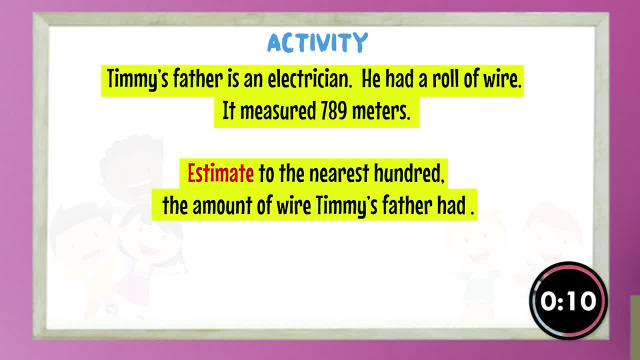 Bake in the oven and heat the food with hot��릴 Roast eggplants. You should be finished by now, So let's see what you have. Let's look at the number centers. eight-nine: We check the numbers of the particularly rounded stomach, So we are rounding to the nearest hundred. eight hundred. 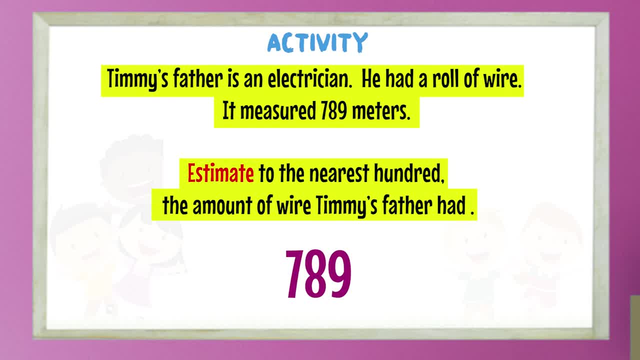 Let's see in this mass with three conditional numbers, If you can't, How many times per secret number: seven hundred eighty-nine, I don't know, I had figures that died. H predict an example to so and so Re Current functions: number seven hundred eighty-nine. 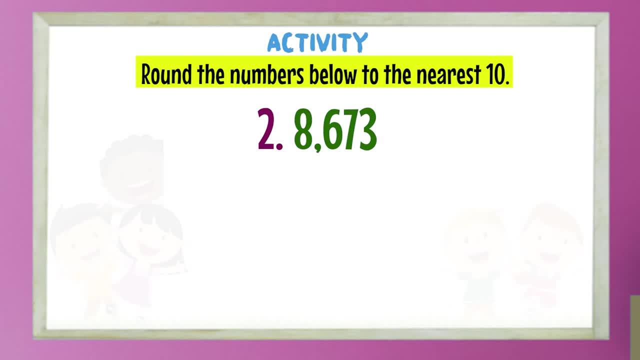 Let's look at the other one. Eight thousand six hundred seventy-three rounded to the nearest ten. Let's add it. Let's identify the number we are rounding to The nearest ten. The number in the tens place is seven. Which number is to the right of that number or which number is hitting the back door of that? 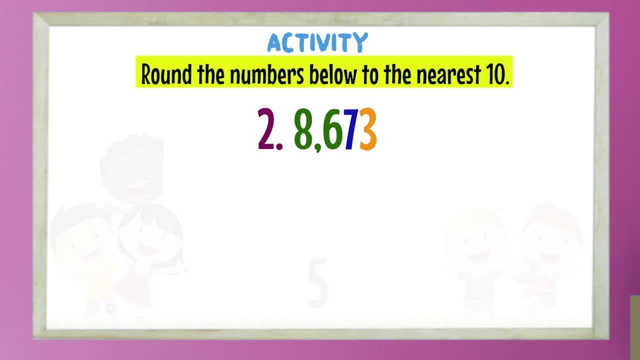 number Three. Is three more than five or is it less than five? Three is less than five. We learned that if the number in the ones place is less than five, we rewrite the number as is and change the number in the ones place to zero. So we write back our eight, our six, our seven and we change. 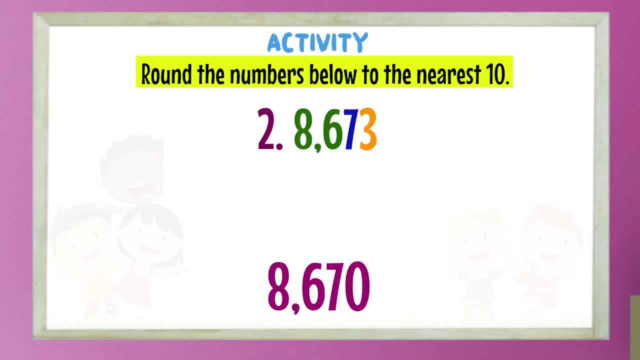 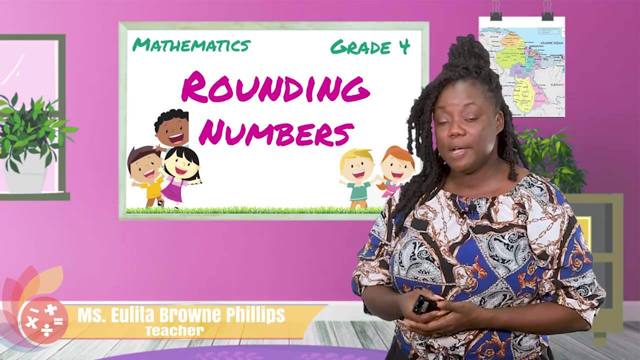 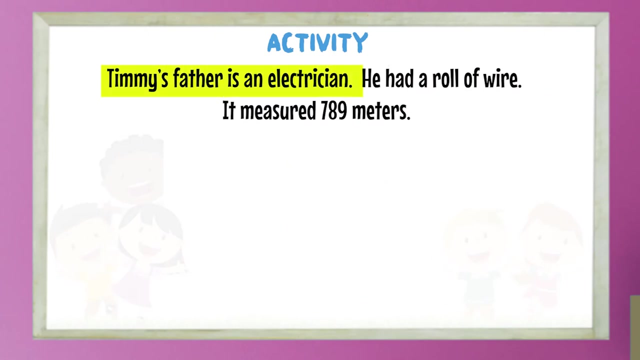 the three to zero. Eight thousand six hundred seventy-three. rounded to the nearest ten is eight thousand six hundred seventy-three. Boys and girls. there is one other activity I want you to do, but this is in the form of a problem. Timmy's father is an electrician. He had a roll of wire. It measured seven hundred eighty-nine meters. 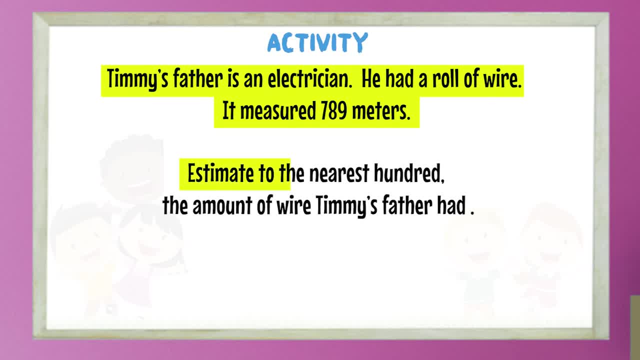 Estimate to the nearest hundred the amount of wire Timmy's father had. What did Timmy's father do, Boys and girls? did you notice I used another rounding word: Estimate. All it simply means is that you have to round seven hundred eighty-nine meters. 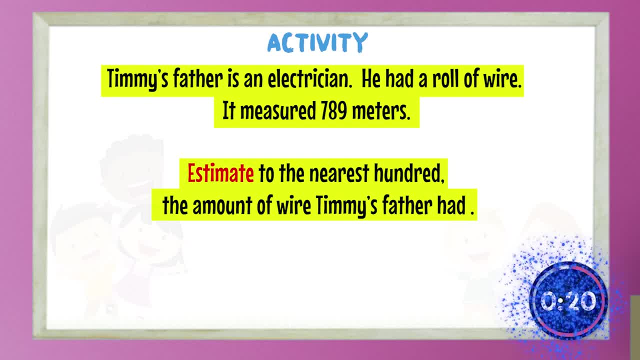 to the nearest hundred. Ok, follow my fraction and you'll get the answer. Now you over, Casey. are you ready? You should be finished by now. Let's see what you have. You should be finished by now. Let's see what you have. 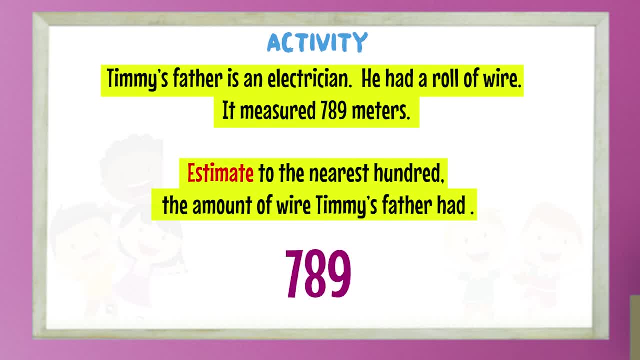 Let's look at the number 789.. Let's identify the number we are rounding to. We are rounding to the nearest hundreds. Seven is in the hundreds place. What number were you around to? What number were you two around to? is hitting on the back door of that number. it is the number hitting on the. 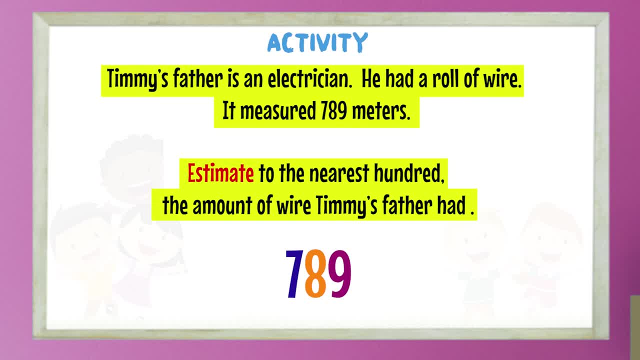 back door of that number. we learned that when rounded to the nearest hundreds, we look at the number in the tens. please, it is in the tens, please. the rule. say: if it's five or more, you add one to the number in the hundreds, please, and change the number in the tens and ones, please, to zero. therefore, 789 meters rounded to. 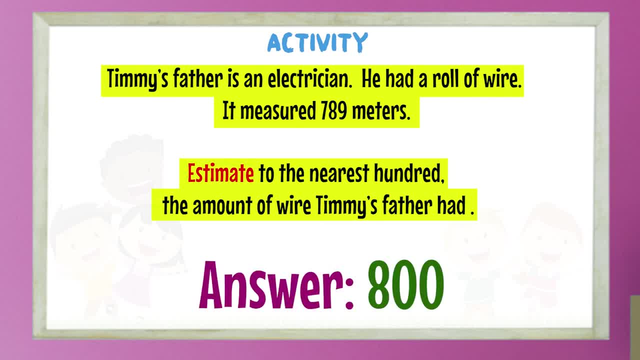 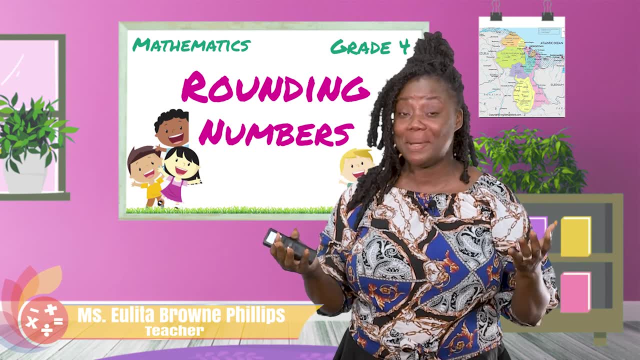 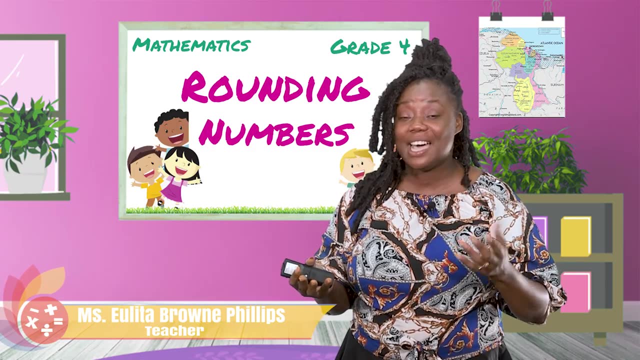 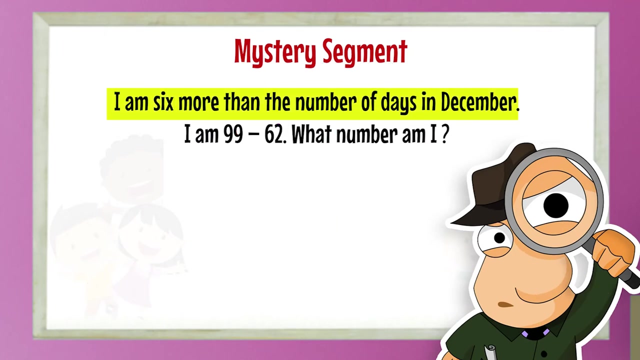 the nearest hundred is 800 meters. boys and girls, it is time for you to solve a mystery in our mystery numbers segment today. look at these clues and solve the mystery. I am more than the number of days in December. I am 99 minus 62. what number am I take? 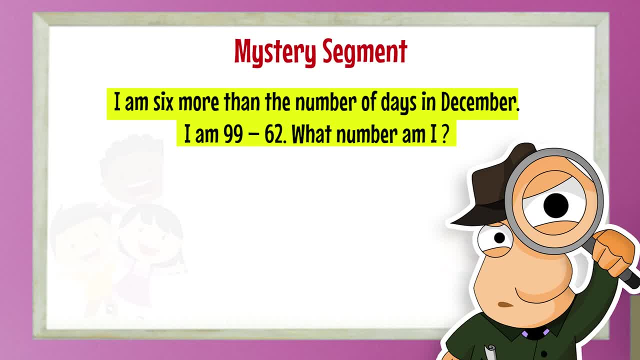 30 seconds to complete this boys and girls mission. you should be finished by now. let's see if you got that mystery. saw the first clue said I am six, three more than the number of days in December. How many days are there in December 31.. 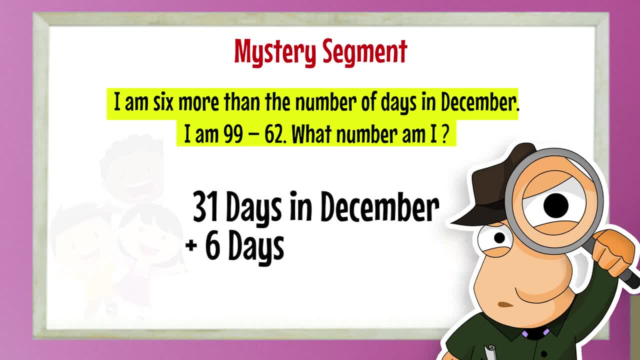 The number is 6 more, so we had to add 6 to 31.. If we subtract 62 from 99,, we will get a total of 37. So the mystery number for the day is 37.. Excellent, boys and girls, Thank you so much for solving that mystery. 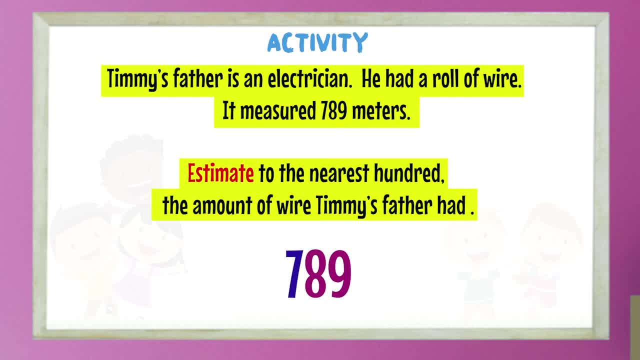 to Seven is in the hundredths place. What number is hitting on the back door of that number? Eight is the number hitting on the back door of that number. We learned that When rounding to the nearest hundreds, we look at the number in the tens place. 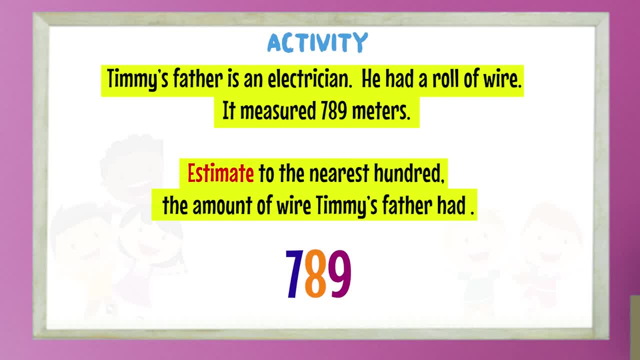 Eight is in the tens place. The rule says if it's five or more, you add one to the number in the hundredths place and change the number in the tens and ones place to zero. Therefore, 789 meters rounded to the nearest hundred is 800 meters. 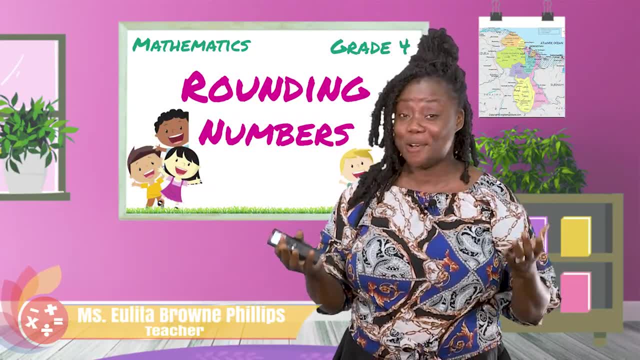 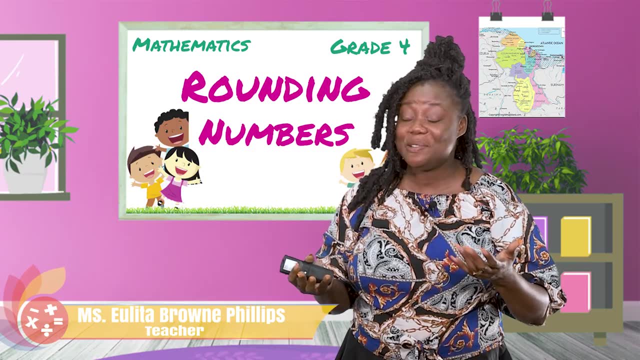 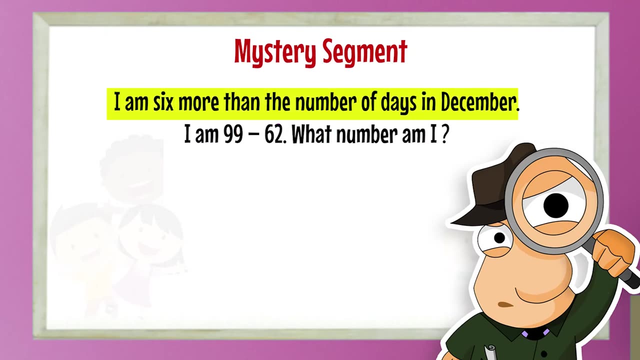 Boys and girls, it is time for you to solve a mystery In our mystery numbers segment today. look at these clues and solve the mystery. I am six more than the number of days in December. I am 99 minus 62.. What number am I? 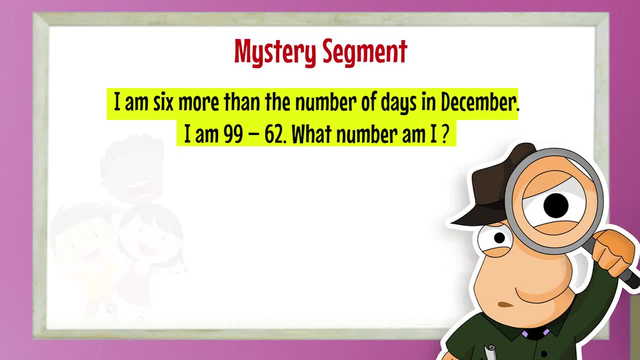 Take 30 seconds to complete this. boys and girls, write a�, then take of three to two equal numbers and divide that into three parts. How many points are like this? What number? Three, Four, Five, Three. What number? 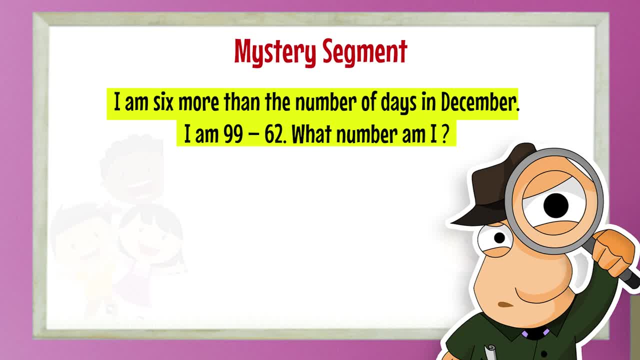 10.. You should be finished by now. Let's see if you got that mystery solved. The first clue said: I am 6 more than the number of days in December. How many days are there in December 31.. The number is 6 more, so we had to add 6 to 31.. 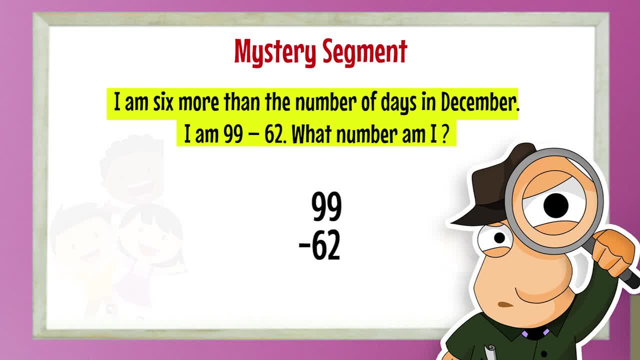 If we subtract 62 from 99,, we will get a total of 37. So the mystery number for the day is 37.. Excellent, boys and girls, Thank you so much for solving that mystery. Now we have to bring the curtains down on our lesson today.